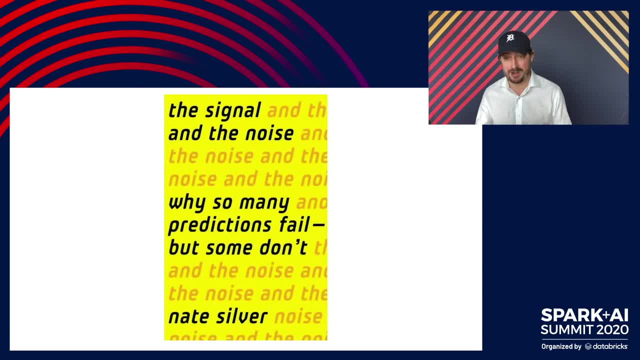 It also took four years to write the book And of course, I had a lot of experience working in analytics before writing the book and collecting stories of the book, with my own research for FiveThirtyEight, and the book and projects before and after that. So, given that we're 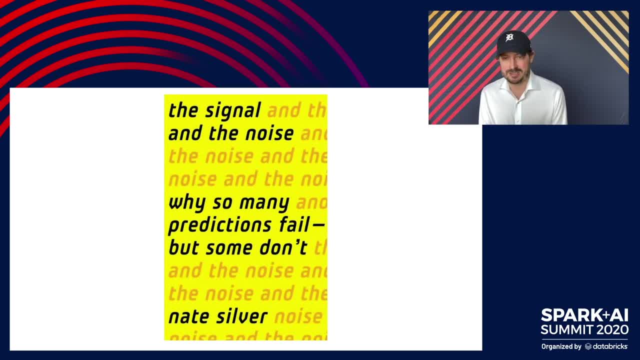 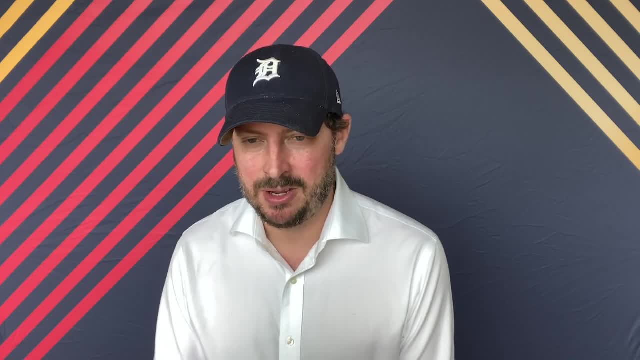 now, in a time of such profound uncertainty, or so it seems, I just want to spend this presentation reviewing and kind of reflecting where we stand in the field of data analytics, And in fact the themes are very true to things I talked about in the book eight years ago. 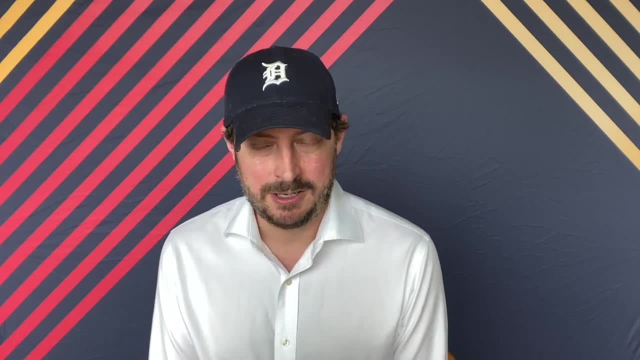 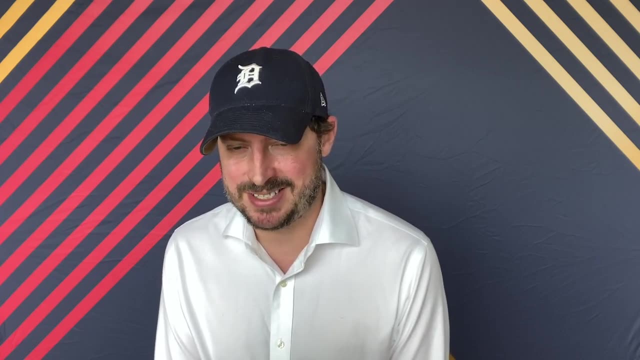 I'm not saying the big picture. things have changed very much. but in light of politics, in light of coronavirus, in light of everything else, I think it's always useful to take a fresh perspective and see kind of the tension between how things look in theory and kind of how things look in. 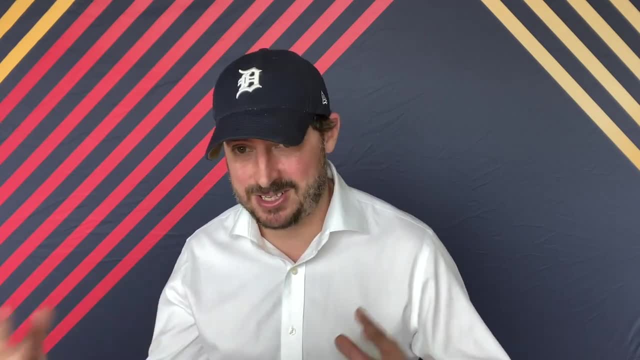 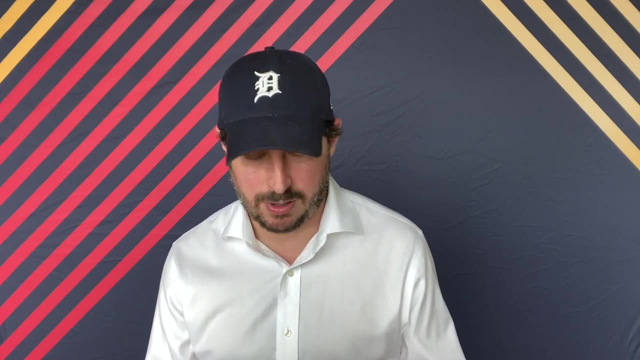 reality on the ground. It's not all going to be coronavirus and politics. We're going to have a few fun stories about sports and poker and things like that. But I do want to increase the focus to you on, kind of, some of the more pressing things that we see today. 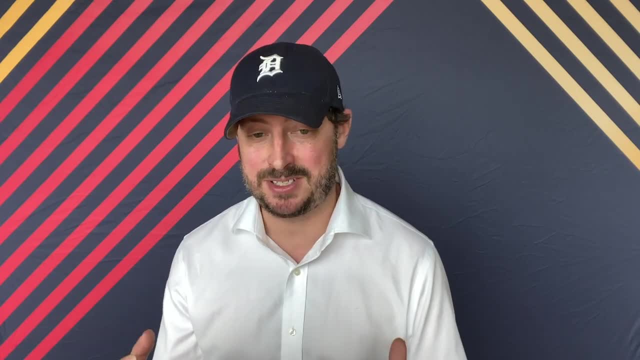 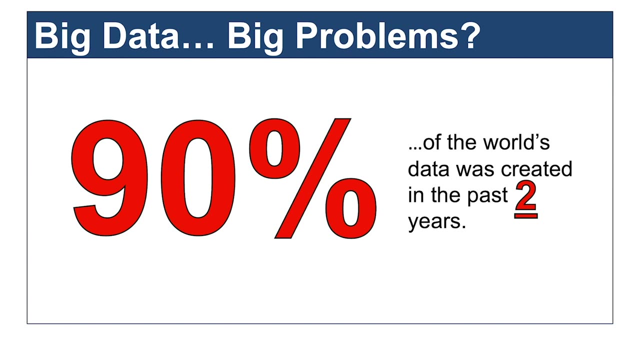 One of the basic contrasts really is between kind of the big promise of big data and analytics And kind of if you were in 2012,, people were very excited about, oh, we kind of can press a button and write a program and we can kind of solve all these problems right. 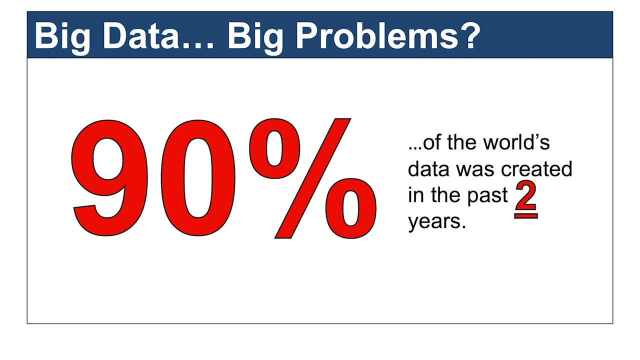 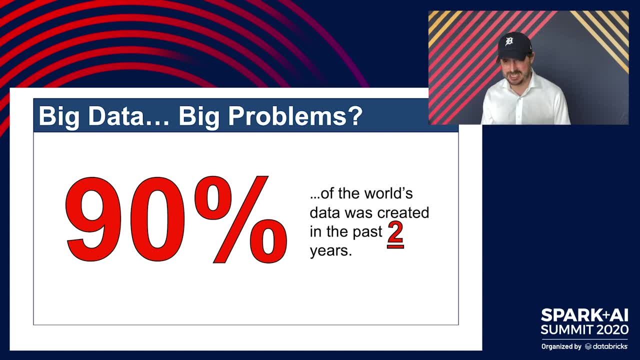 You would hear a lot of statistics like this is from IBM, for example, that 90% of the world's data at any given time has been created in the past two years. That sounds like great right. We're solving all these problems, except if you think about what's kind of happened over the past. 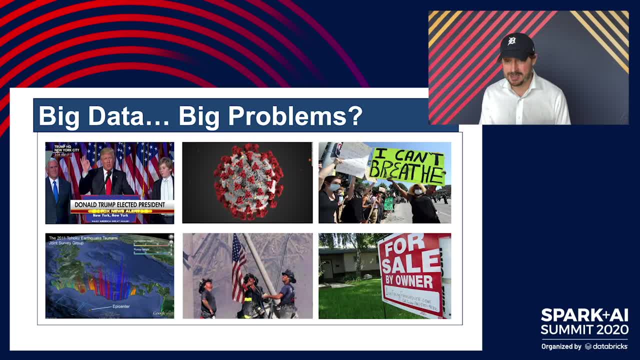 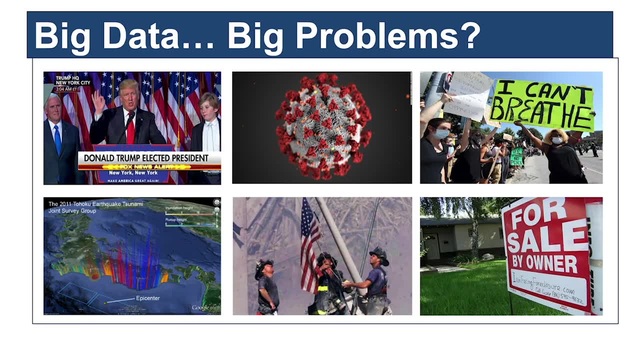 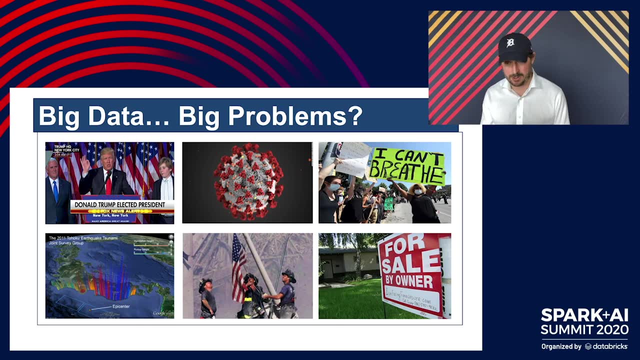 decade or so it's been a lot of things that were problematic or unpredictable or both, right Ranging again from elections to coronavirus here in the middle of the worst pandemic since the Spanish flu. You also have some of the biggest protests arising in the US since. 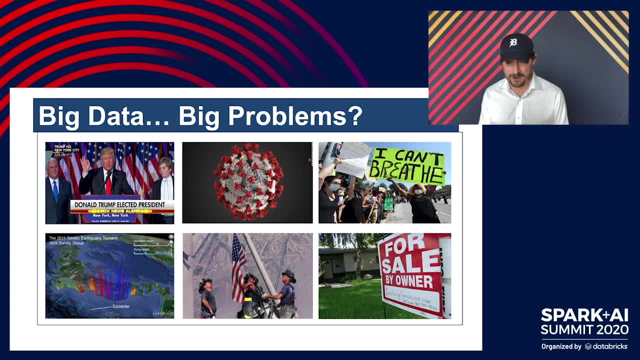 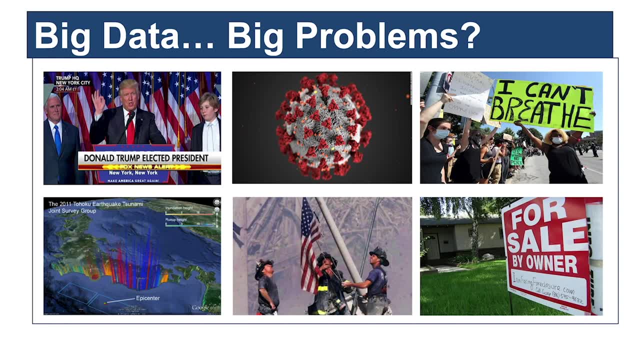 1968.. We have also all the stuff that goes on in the background, like earthquakes and the recession right now and terrorist attacks and hurricanes and all that stuff. I would recommend, by the way, if you want to read the book. we talk about almost all these things in some detail in the book. 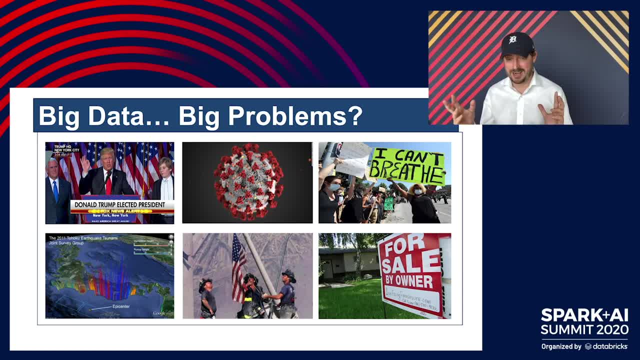 But the contrast between the promise that we think the data creates and the fact that the world doesn't seem to be becoming more predictable, I think, is something that we need to confront a little bit more head-on potentially. By the way, it's not just these big newsworthy. 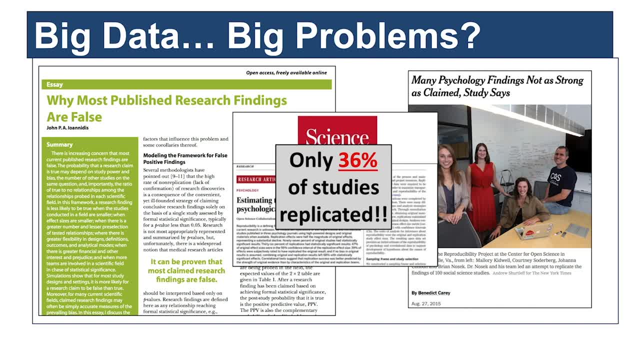 events that can create tension and surprises and problems. It's also in some of the most scientifically minded fields of all, like medicine, for example, or psychology, where only about depending on which study you read, only about the big news that you read creates a bunch of big. 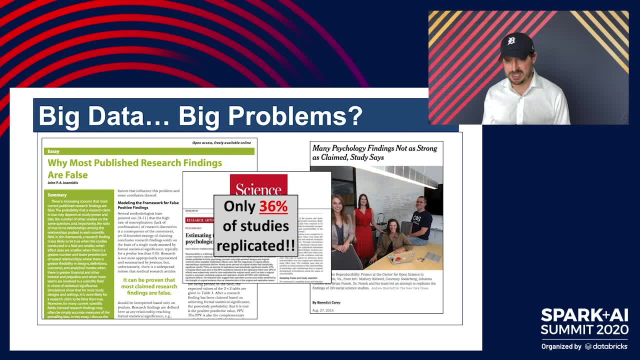 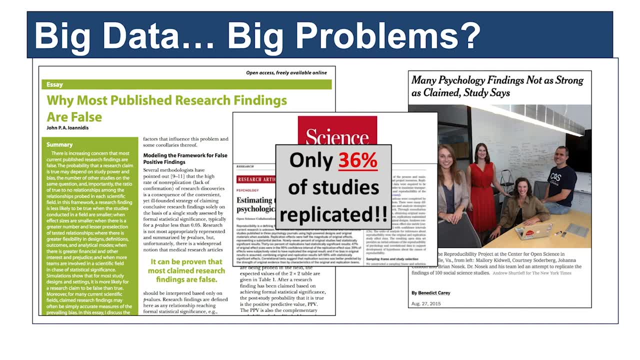 about 35 to 40 to 50 percent of scientific findings can be successfully replicated, meaning that you publish a result in a journal. you say it's statistically significant. we have a big discovery. another researcher tries to recreate the same finding and they actually fail to do that. 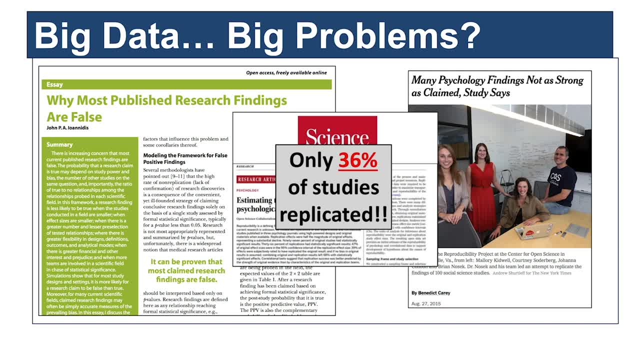 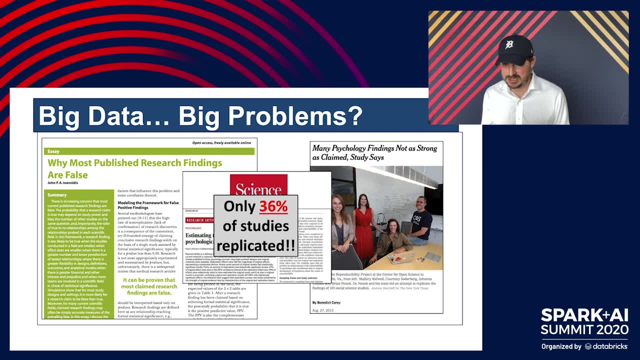 as often or more often than not. So why does this occur? This is a big problem, for example, when you read all these studies around coronavirus treatments and vaccines and things like that, where there'll be some promising initial discovery, whether it's about a therapy. 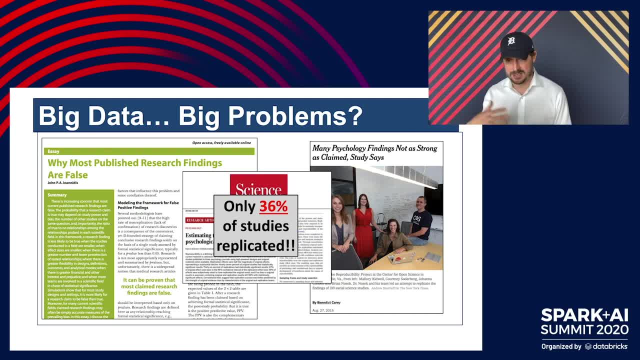 for example, or it might be about, if not a therapy, then some hypothesis about how the disease might spread. Maybe it's indoors and not outdoors, or maybe it's aerosols or whatever else. But you'll find that sometimes these findings aren't robust when people go back. 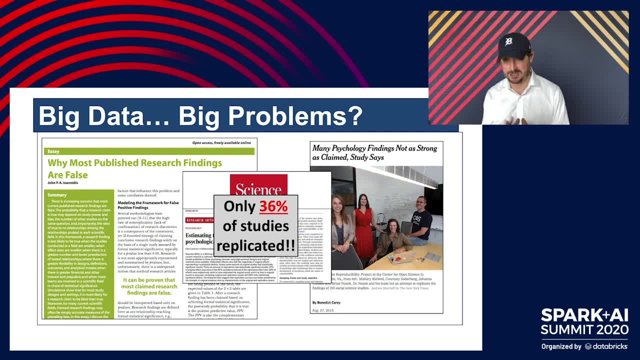 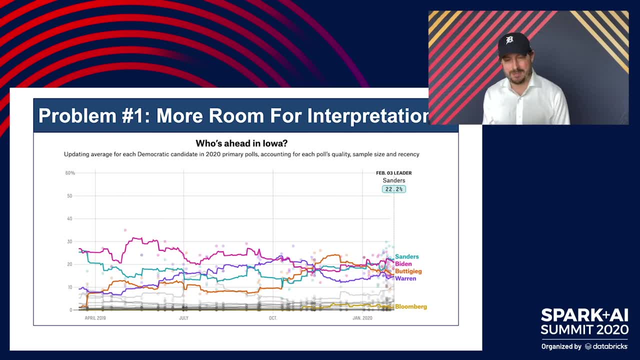 and look at them again. So I will try in this presentation to talk about why some of that can occur. So one thing I think people don't think about very much is that when you're in a disease study, you're going to have this beautiful 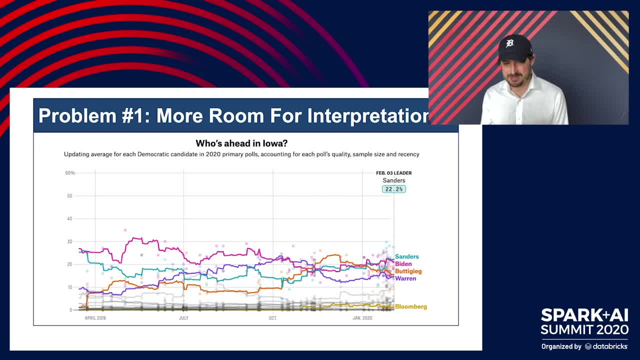 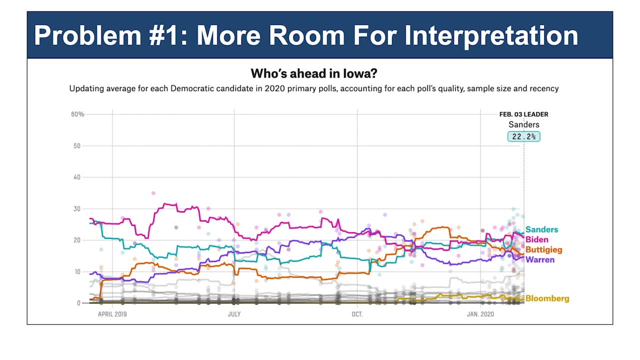 henny-like, and you're going to have all these attributes. you're going to have this. you gather more data, um. that actually leads sometimes for more room for interpretation or disagreement, right? Um? it used to be that. um. in political analysis, my specialty is looking. 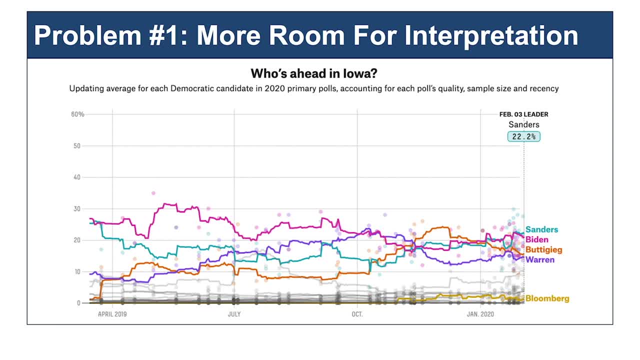 at political polls forecasting elections. It used to be that, hey, 30 or 40 years ago, you would have a few big national polls. You'd have an NBC poll and a CBS poll, the New York Times poll, the ABC news poll, right Um, you would have maybe a few high quality state polls. 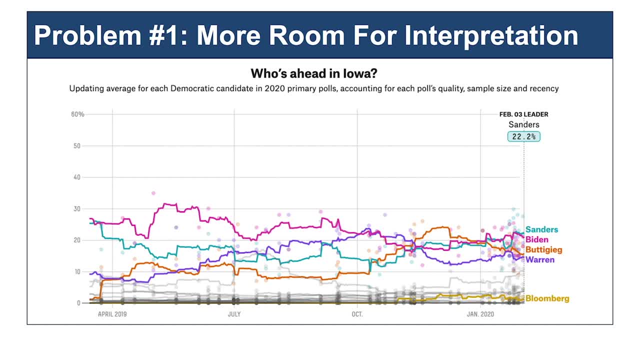 in in Ohio or Iowa or whatnot. Um, but you didn't really have nearly as rich the amount of data that we have today, which, on the one hand, seems like, oh, it's really disappointing, right, We can't have as much precision on how we look at every swing state and make these fancy. 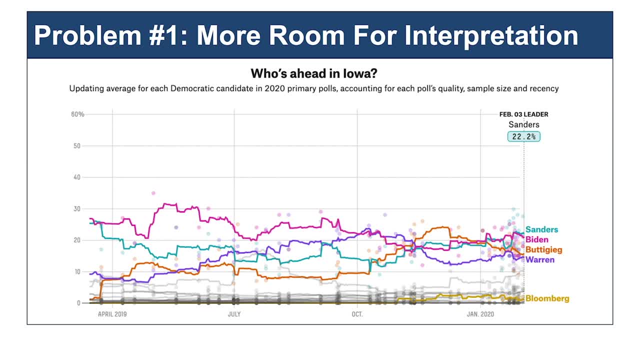 maps Sites like 538 couldn't really work very well. You barely have polling in many states, right Um. on the other hand, when you have lots and lots and lots of data, then there's lots of room to argue about it, potentially Um. here, for example, is our chart from 538 showing what the 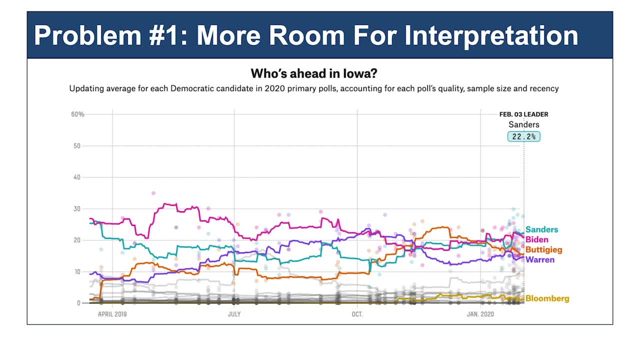 polls show Over the course of the Iowa caucus: um, we spent a lot of effort to figure out how much you want to smooth the data and how you want to kind of literally connect the dots. Um, even so, you had, in Iowa at some point, four different people actually led the Iowa caucus at some point in. 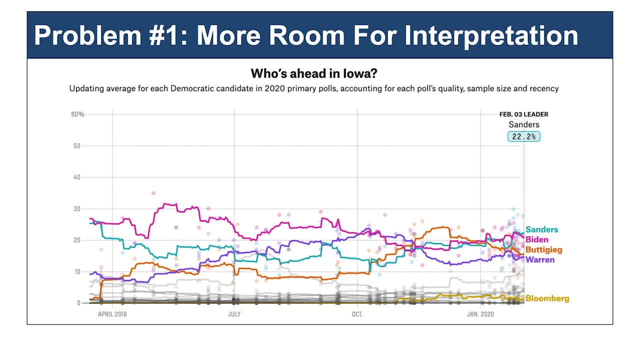 the polls, It turned out you basically had two different winners, to add to the confusion, where Bernie Sanders and Pete Buttigieg- each one Iowa, depending on exactly how um which metric you look at- the state- at least three different counts of the vote to make things even more. 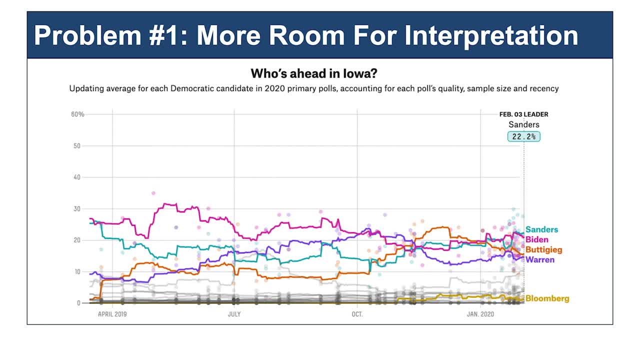 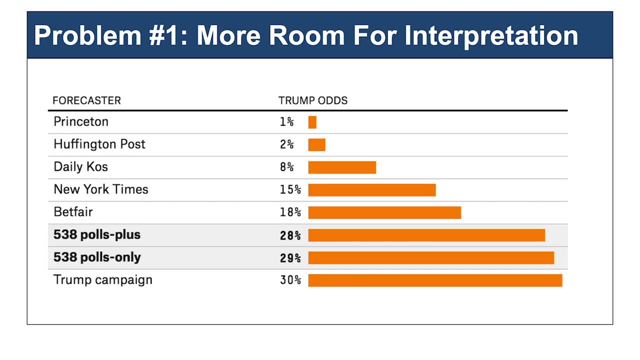 confusing, So um so it certainly doesn't seem like, as we get more data, that we've achieved more consensus. There's actually as much fighting and arguing and room for debate as ever before. And if we go back to 2016,- the general election- there was a lot of controversy over election. 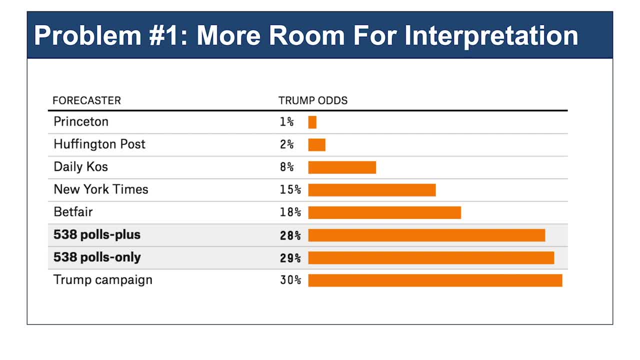 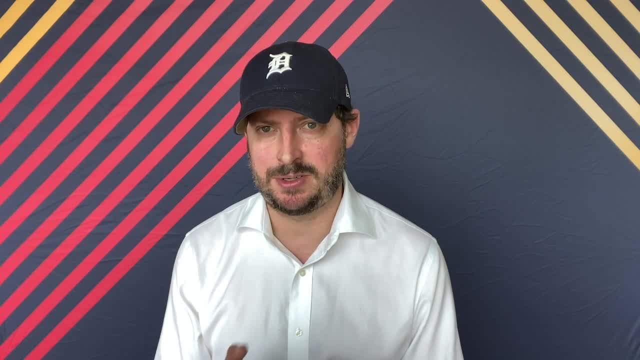 forecasts. Um. what is important to note, though, is that you actually had people taking the same information, the same data. all of these forecasts are looking at polls and sometimes economic data, but mostly just at polls, and coming up with very different answers. Um. 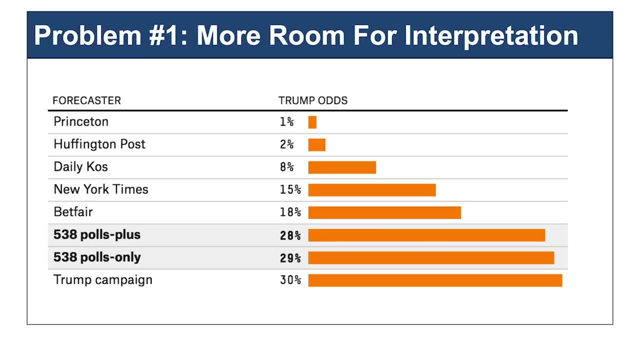 we're. our forecast at 538 gave Trump about a 30% chance of winning Um. the Trump campaign itself allegedly also gave itself a 30% chance of winning Um. the other forecast gave him only a 1% chance or a 2% chance And to me, working in probabilities, a three in 10 chance, or one in three or one in. 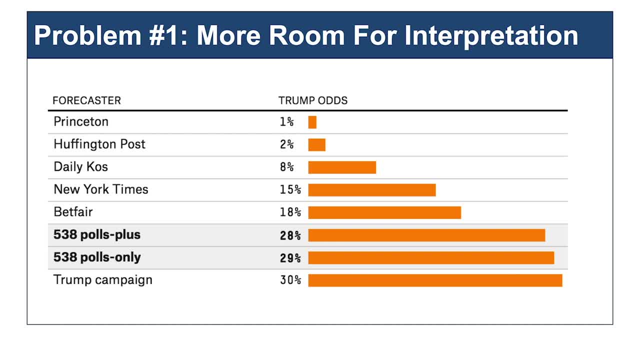 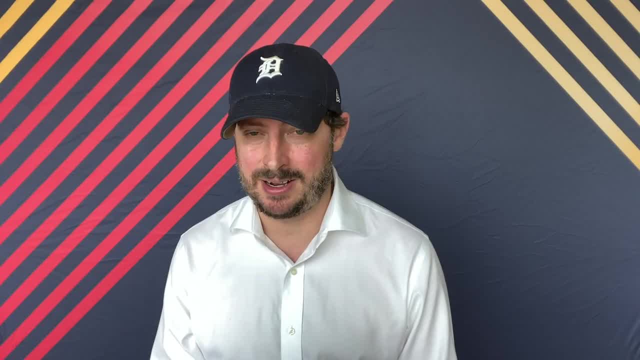 four, whatever you want to call it, is very different than one in 50 or one in 100.. Um, so the kind of romantic notion that, Hey, if we get all the data that we need, um, and that's the easy part or that's the hard part, solved right, It's like no, actually the hard. 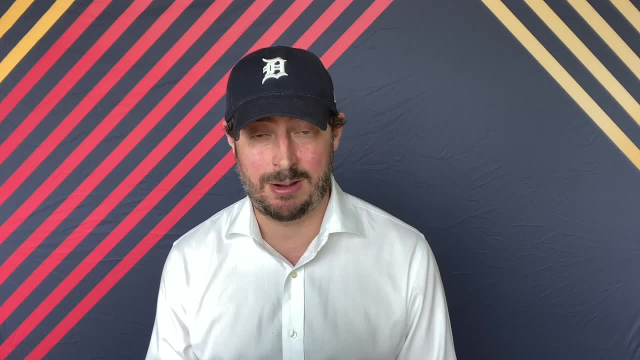 part's in the actual analysis. The hard part is in the modeling. Often the hard part is in how you account for uncertainty right. We can all look at the polls and say a certain candidate is ahead by three points. Um, but how big is that margin of error? Is that margin of error? 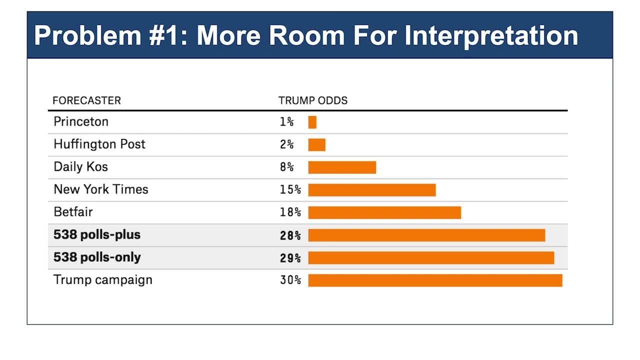 symmetrical or are there funny shapes to it and whatever else? how are different states related? Um? you know Wisconsin and Michigan and Pennsylvania, for example. those all went through Trump in 2016.. Well, those states are all really correlated, as we call it Um, because you have the 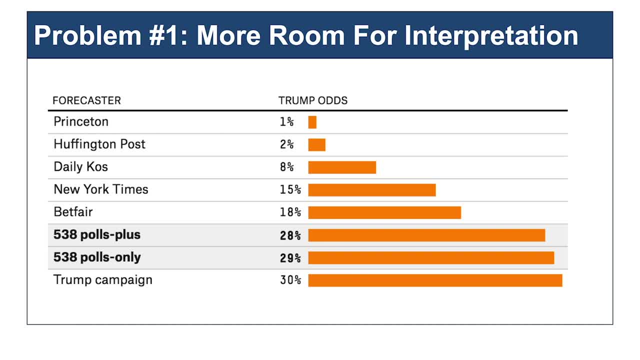 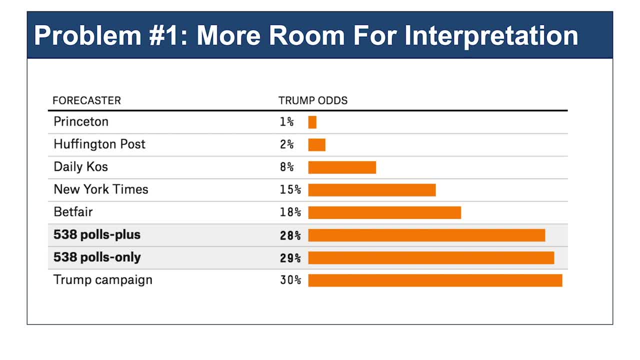 odds and others was because we understood how these states are not independent. You do not actually have 50 separate states voting at once. You have um people voting all across the country and 50 manifestations of that in different parts of the country. Um, of course, like I said there, 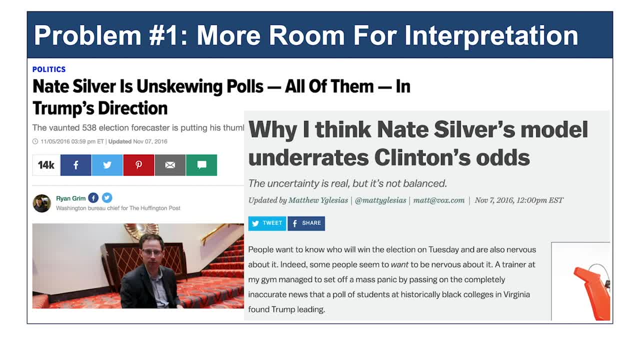 is a lot of second guessing, as we're having new election 2020 coming up soon. In fact, I'm kind of um working on my 2020 model right now. It's kind of what I'm spending most of my time on as we speak. Um, but there was kind of a real um, a real shift in perception before. 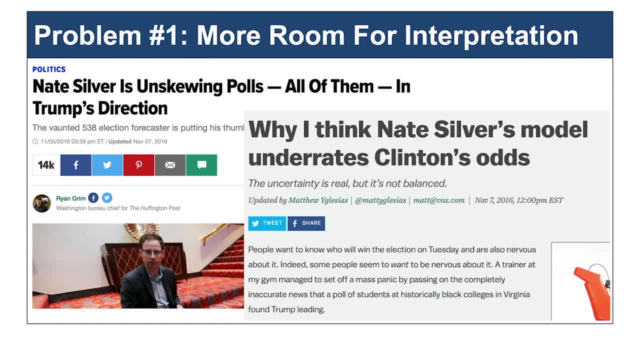 and afterward, where, before the election, people were surprised that we had Trump so high, Of course, after people thought, well, why didn't you have Trump winning? Um, there's a lot of second guessing- if you've ever been, of course, as most of you are practitioners in analytics. 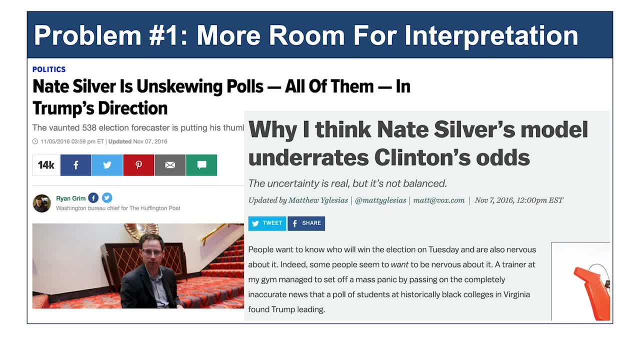 people are really kind of results oriented and not process oriented. I think thinking more about your process is more important. If it's more about probability is important that if you have any forecast saying something should happen 30% of the time, it actually should happen 310 times. 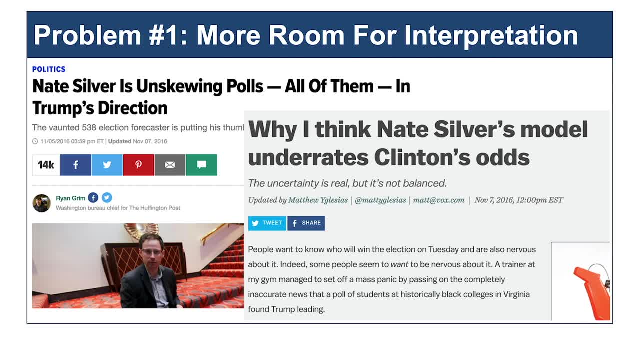 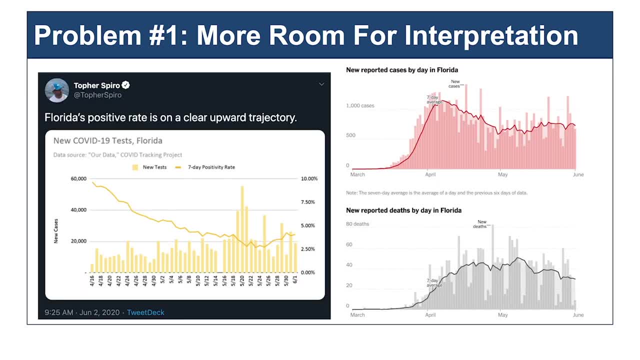 like a flush draw in poker or something that's supposed to happen some portion of the time, Um, but I won't dwell too much on on 2016, when we have so much other news to cover. Um. you also see, though, when it comes to coronavirus, a lot of debates over how to 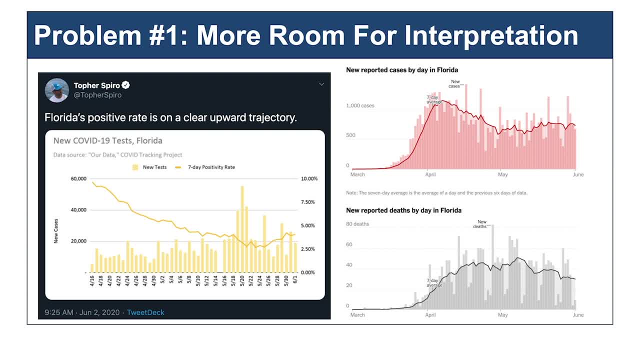 interpret different data, And it does remind me a lot of polling, where one of the things about this is you have 50 different states and then you might each have five or six different polls per week. You can look at different versions of those polls, right, So there's lots of room to kind of. 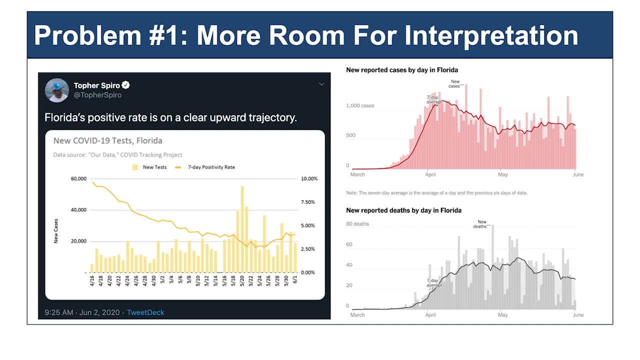 cherry, pick your way toward any narrative that you want within within some degree of reason. Um and likewise. here you see, for example, you see lots of tweets like this- that Florida's positive rate is on a clear upper trajectory. You know, to me I'm not sure if it's clear or not. 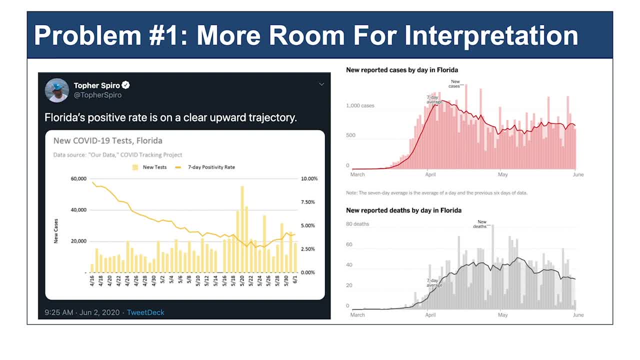 Um, here's some graphs from the New York times. looks at deaths in Florida and reported cases in Florida As of now, a few weeks ago, if you're watching this in real time. um, the point is that, like we're just trying to find more and more ways to argue- I am not 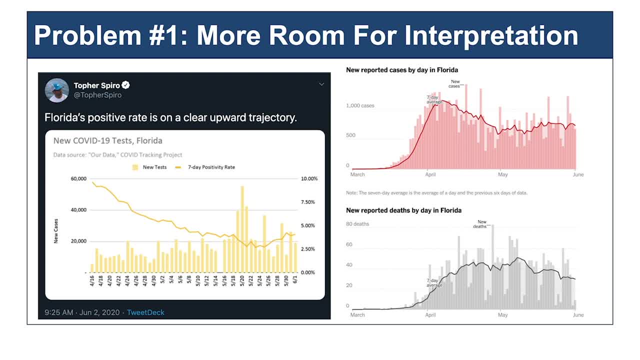 a postmodern relativist or something. I am not saying that there's no absolute truth. What I'm saying is that motivated reasoning, um is a big issue, um, where we have things that confirm our priors, whether they're partisan fires or whatever else, And that can make us 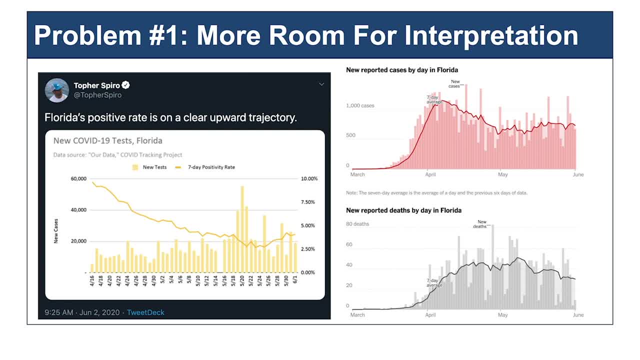 um less inclined to accept more nuance and uncertainty, um less inclined to understand, when you know, by the way, part of being pro science, understanding behavioral science and how we are people who love to find things that that tell us a story that we want to hear- that confirmation bias is really quite powerful. 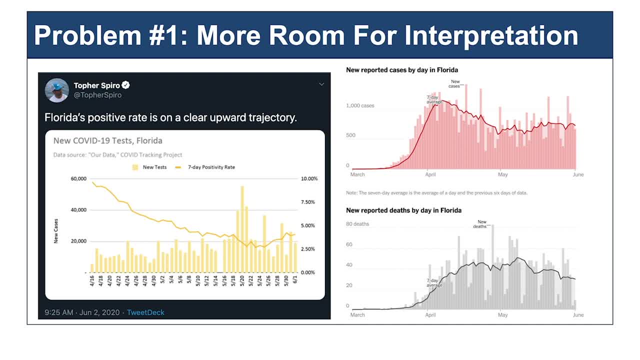 And kind of. the longer I've been involved in covering politics and making forecasts and looking at data in a very, very public facing way, the more I think people are getting worse and worse about having their beliefs and their priors confirmed and not realizing that they too 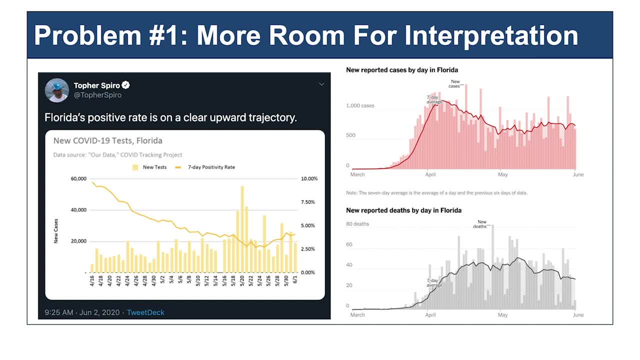 no matter how smart you are. that's often experts, smart people, who are more prone toward um creative interpretation of the data that might fit their, their beliefs. Um, you have to be really, really careful and rigorous. Um. issue number two is the way in which complexity tends to increase as you increase the amount. 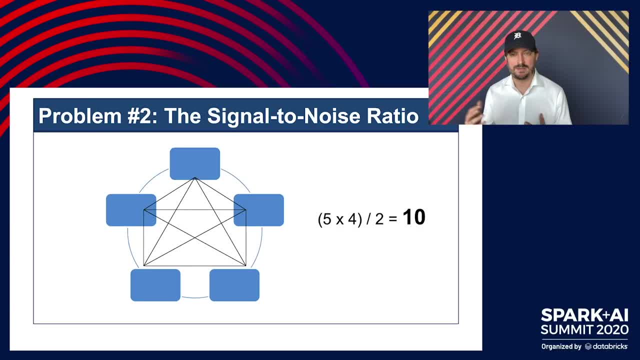 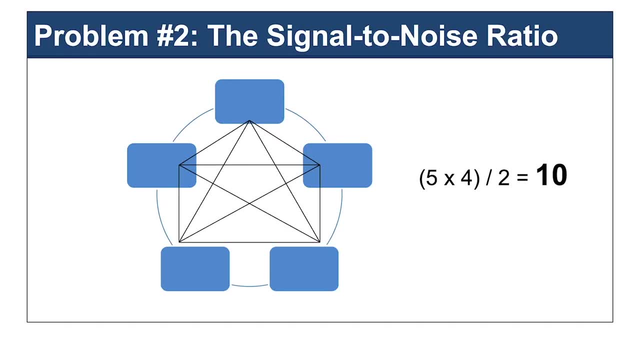 of data in the world. Um, so if you imagine that you have just five variables, for example, you're trying to look at the relationship between, say, inflation and GDP grow- Um, well, there are 10 two way combinations of variables that could run tests on, for example. but but what happens when? 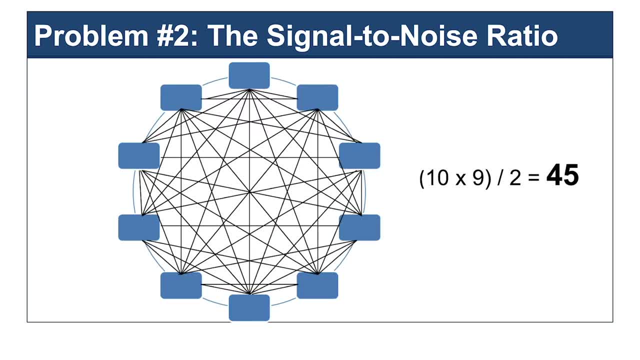 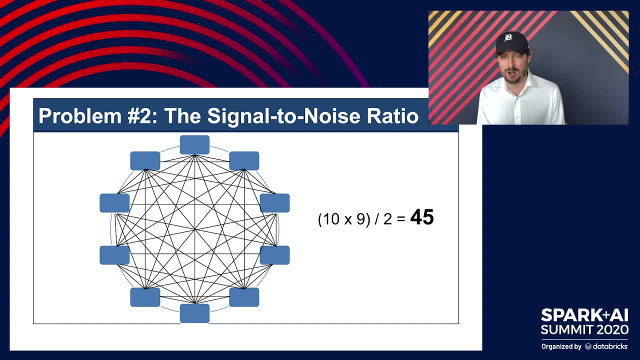 it begins to expand, say, instead of five variables, you instead have 10, when you start to see a geometric increase in the complexity of relationships, Um, it's a bit like a um, a meeting or, I guess, a zoom call. now, right Where, um, if you go from having five participants to 10,? 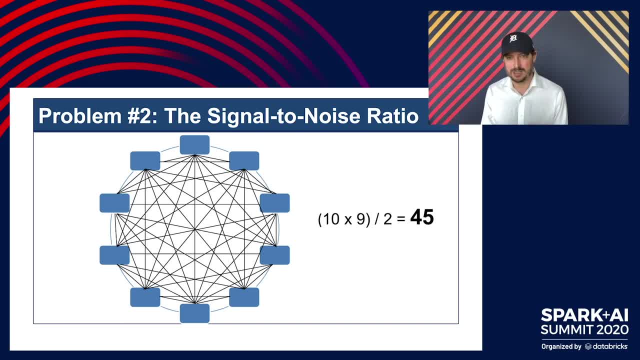 the amount of chaos increases kind of an exponential rate potentially, um, the amount of tension between two people or the amount that people want to share things becomes a lot more complex. Um, but it's kind of keeps going up where, if you look at economic data, for example, 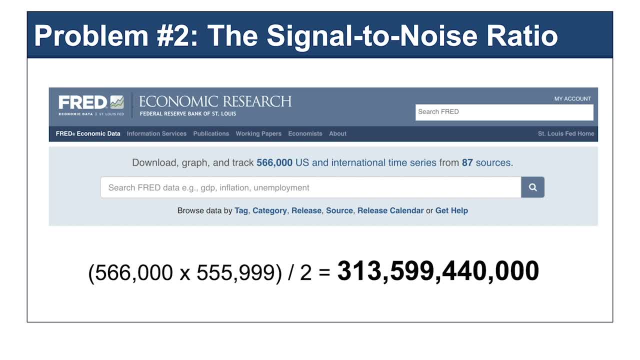 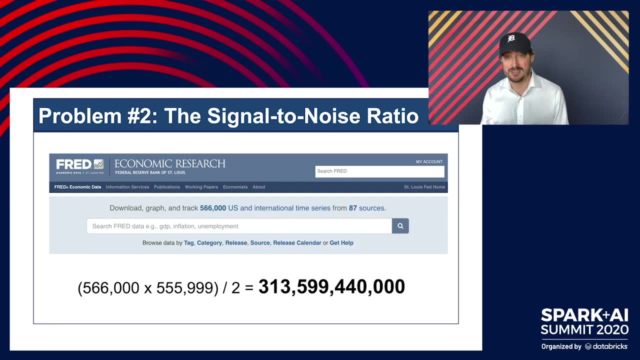 the federal reserve now publishes about 566,000, um uh economic statistics. they update in real time every day. Um, so to look at all possible combinations of those, you would have 313 billion, 599 million, 440,000 possible tests that you can run. Um, and the problem here is that when 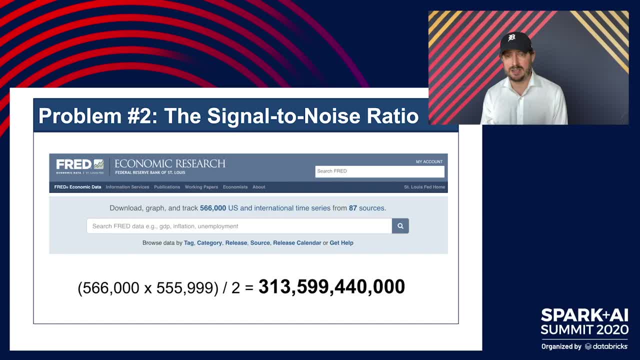 you have kind of infinite or almost infinite amounts of data. then you can find something which is um, which is a one in 1 million coincidence, And you actually find quite a few of those in data sets that are this large. you know, it sounds like a little bit abstract. 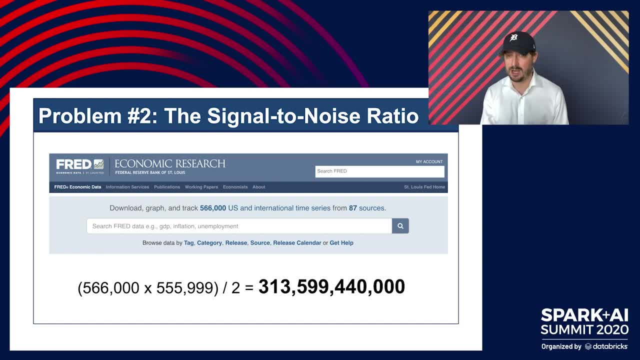 Um. but this gets back to why, when I talked about before about um replication crisis, why do only 35 or 40% of the findings replicate? Well, people will um explore so many possible ideas that they will get very excited about things that happen because of chance alone. 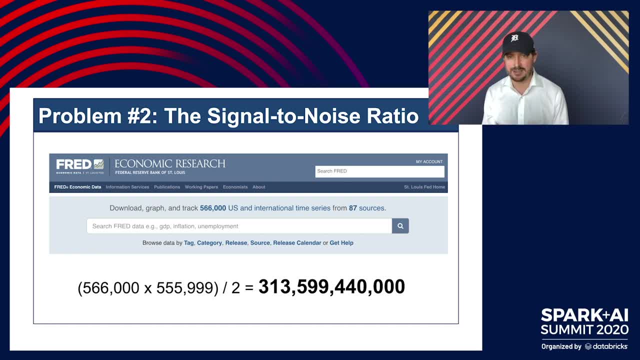 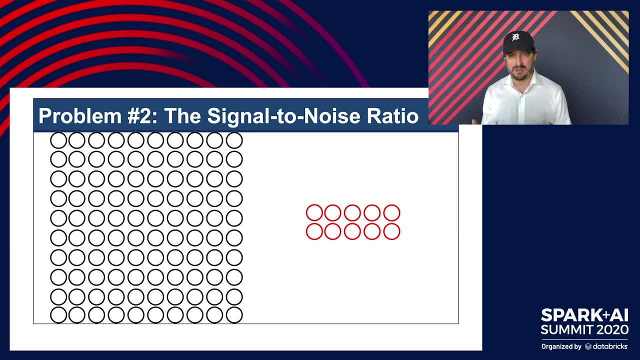 or because of bad data, or because, frankly, sometimes of bad research design, Um, and so there are all kinds of ways to to fool yourself, Um. let me give one more more sort of abstract example here, Um, but it's pertinent in epidemiology and it's pertinent in. 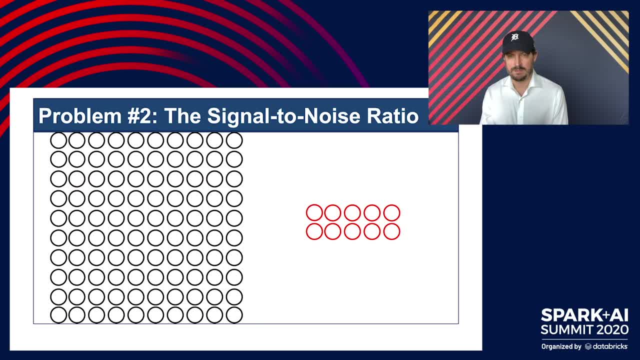 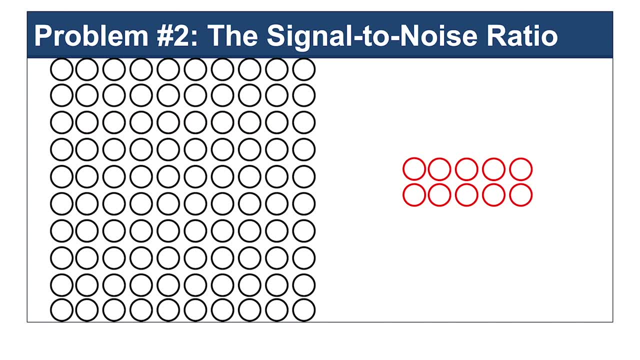 research and a lot of other areas. but so imagine that we're looking for for signals, and by signal I mean something which provides useful information about a relationship. Um, maybe, for example, trying to find coronavirus cases, for example. uh, maybe we're trying to find um, if we're in. 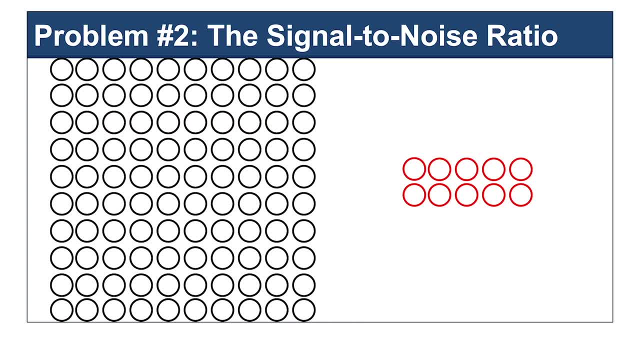 investment, trying to find research strategies that actually work in a robust over the long term. Um, so this depiction: imagine you have, uh, you see, 10 red circles. these are signals and the 10 black circles are are noise. Basically, they are false hypotheses. So okay, But let's say that we 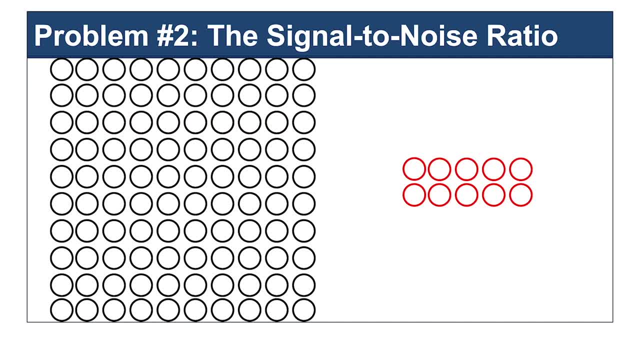 are smart and we have an algorithm, we have our judgment with everybody else, And so we? um, we are able to filter out 80% of the false signals. Um, meanwhile, we are able to capture 80% of the true signals. Um, that seems pretty good, right? We've made a lot of. 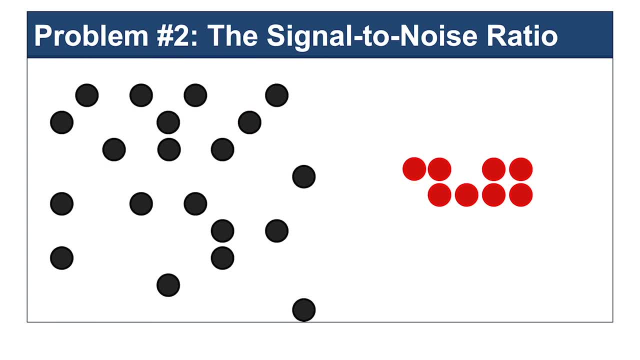 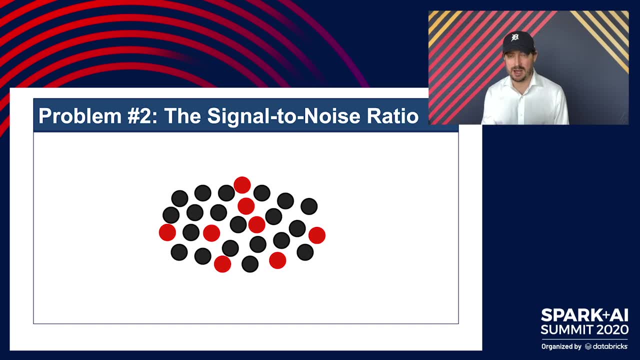 improvement from this kind of very signal poor environment initially. The problem is, if you recombine these because the initial signal was still was still so poor, you still actually have um more false findings- the black ones, than true findings- the red ones, And again. 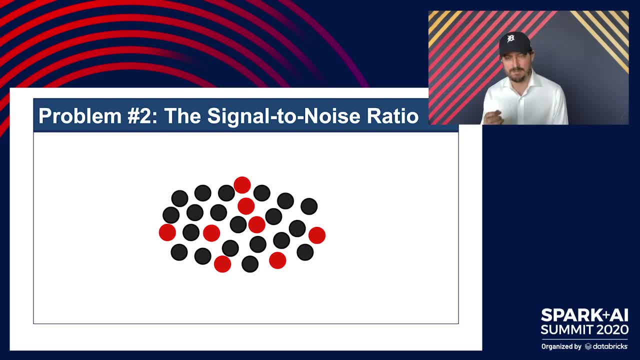 this is pertinent in areas like, um like, diagnosing a disease, where if, for example, you give mammograms to women who are in their forties- fortunately women in their forties are fairly unlikely have a low base rate of breast cancer, for example. So it turns out that 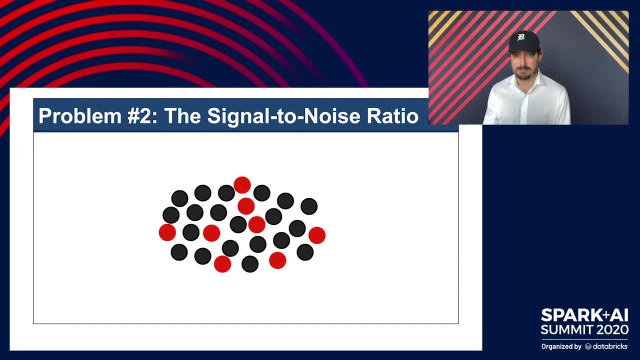 um an initial mammogram if you're in your forties, a woman, and it comes up positive. actually, majority of those cases are false positives the first time. So what you have to do is go through that filtering process a second time and a third time and maybe a fourth. 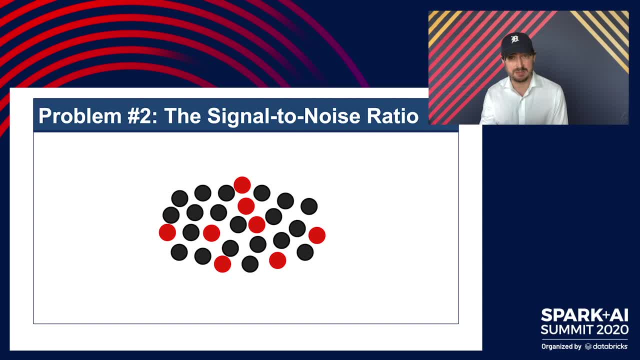 time And then by then you finally filter out enough false positives and different types of tests where you have a more reliable signal. But, um, but this is why you know, for example, in clinical trials for some new vaccine for COVID, um, you're going to read lots and lots of um, very 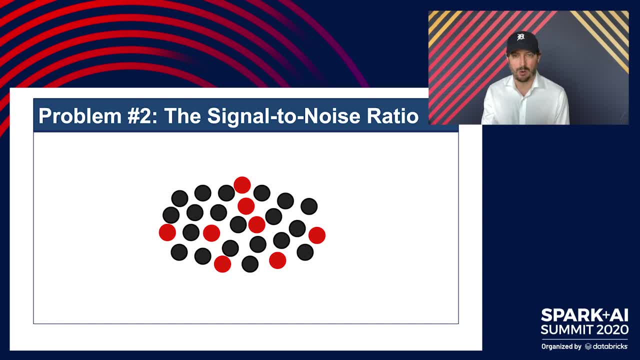 enthusiastic reports about stage one trials, um, or initial promising results from therapies, And the fact is that um- probably the majority of these, maybe the vast majority of these will- will not pan out. um will fail at some phase or another. Now, the good news is that 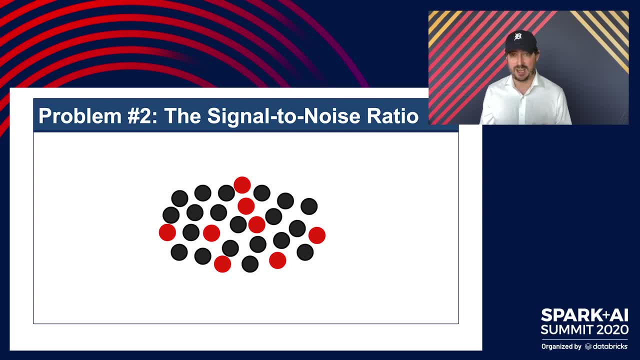 there are so many attempts at doing this, where you are kind of playing a numbers game and odds are also that, of these many possibilities, that some actually will work. you'll learn from the failures as well, Um, but this is important to keep in mind when you're kind of we have a brand. 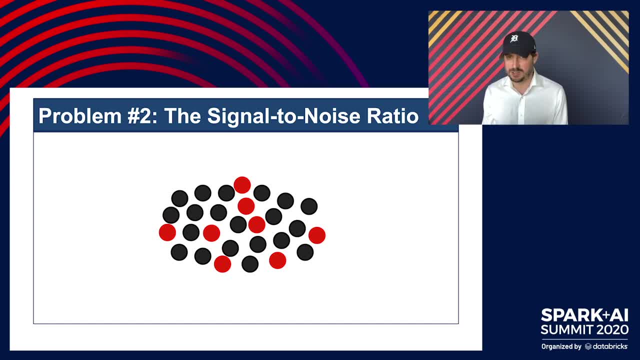 new disease, kind of taking over um the world somewhat literally, unfortunately, um learning a lot more about it. but like, but we are kind of starting from an environment where there's a lot we need to learn and discover. Um, the final problem is what happens when you get in environments. 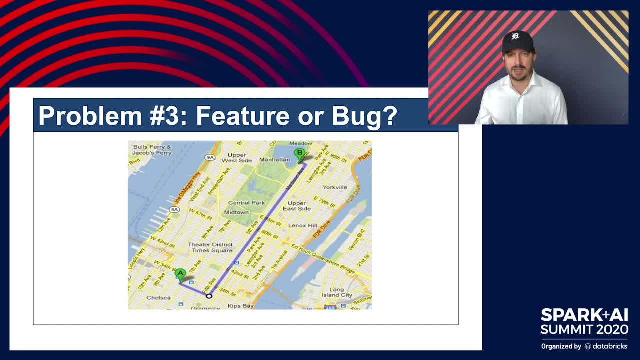 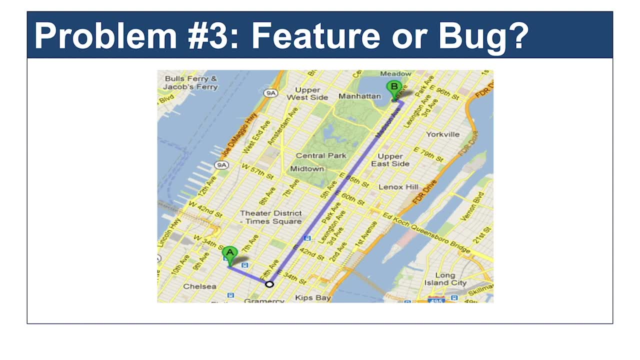 that are competitive, where you have one interpretation of the data and um and other people might have a different interpretation of the same evidence, Um. so an example here that I'd like to give is back from um, back from pre COVID days, when um 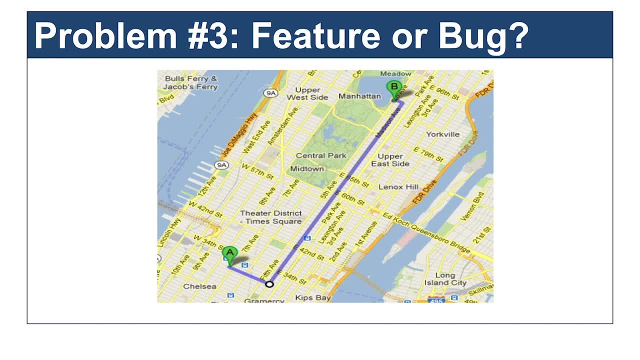 when I was giving a talk in person um at the Guggenheim Museum in Manhattan. you see here where my apartment um is in Manhattan, and how do you get from point A to point B? Well, it would seem like it's pretty simple, right? Um, of course, there's a lot of. 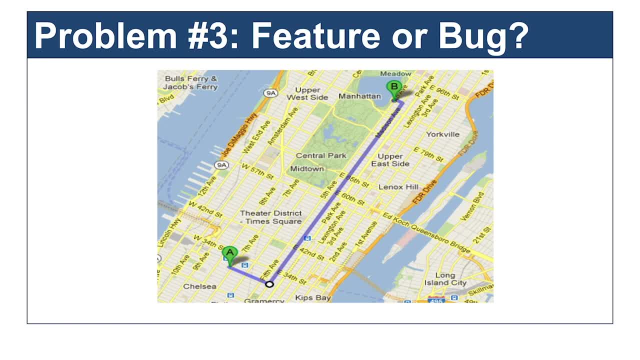 traffic, so it's a slow drive, but basically you just take um a left on Madison Avenue and you drive North for um for 30 minutes or so and then it's pretty straightforward. So that's how you would look at Google maps, how they would get from point A to point B. Um by contrast. 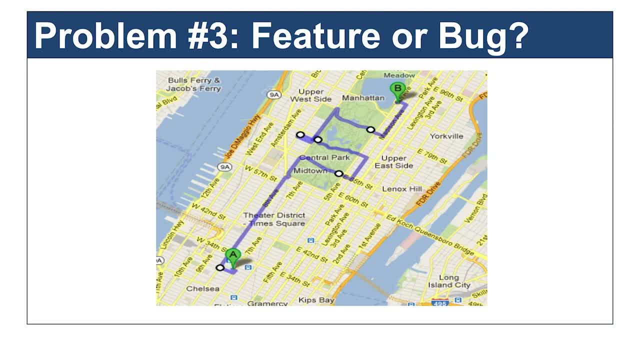 this is the actual route that my Uber driver took that day, So we crossed through Central Park three times to the loop-de-loop at 72nd street or so and finally got to um the Guggenheim about 45 minutes late, Um. so the question is: why was this driver taking this route? This was not a 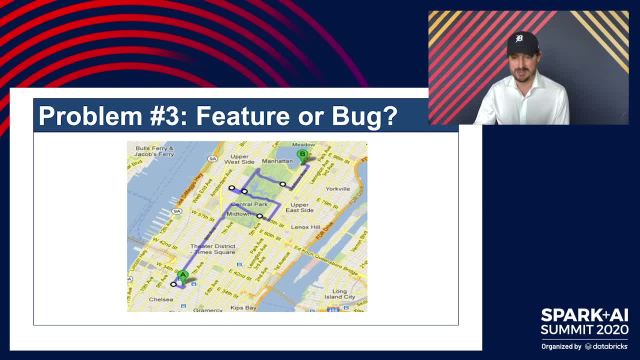 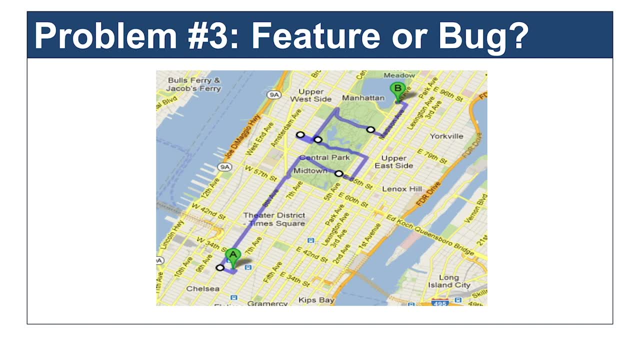 very efficient route whatsoever. You would figure with all these people in Manhattan. you know this is not the way most people would go. Um, well, it turns out that the driver or the GPS, not the driver's fault. it was the GPS's fault, um of the routing software. 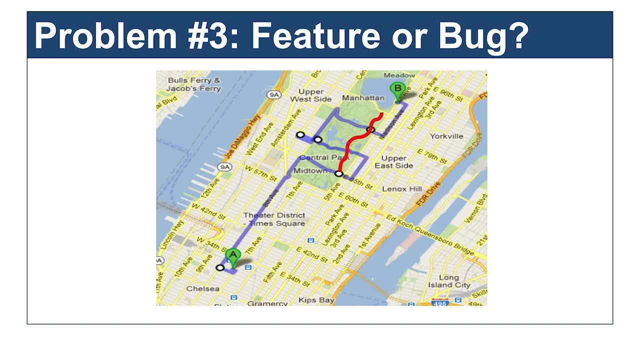 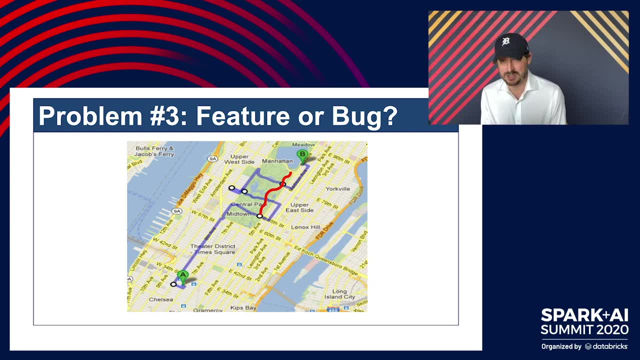 I should say um was very intrigued by this road that cuts North through South, through Central Park, called East Drive, Um. so East Drive is a real road. Most of the time it is reserved for um for people who are biking and jogging, but at certain times of day it's open for through. 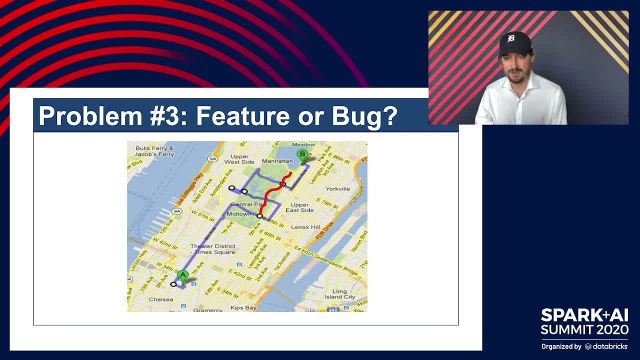 traffic. Um, the problem is that the GPS thought that East Drive was open at 2 PM, or whatever it was, on a Tuesday, when in fact that's what time it's closed, And so it was trying to take advantage of this signal. that turned out to be basically a bad data point, Right, Um? so of course, the driver 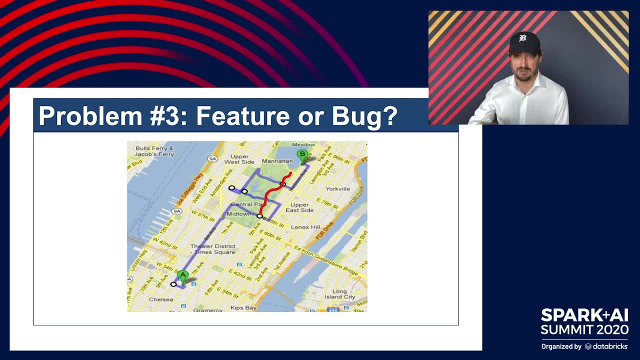 was like: okay, if I can get on this, there's no traffic there, It's a shortcut, I will save lots and lots of time. Um, but very often when you kind of find something that is too good to be true, 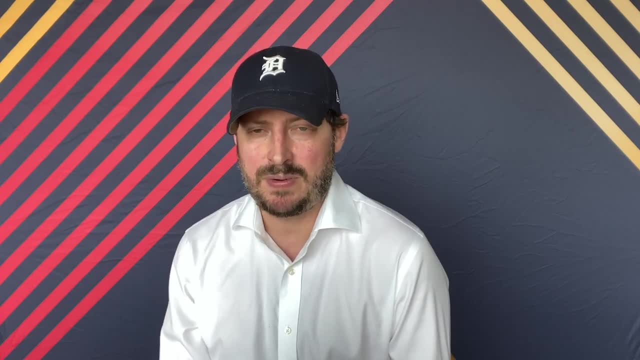 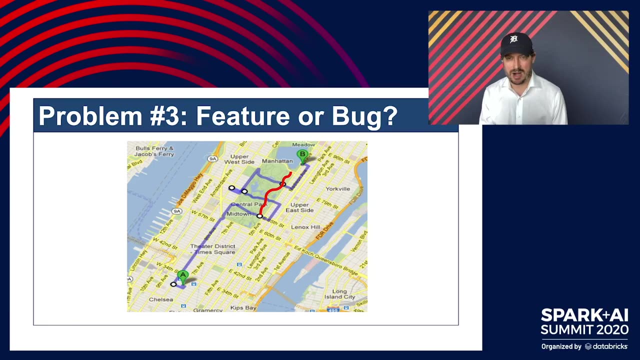 then it actually is this kind of applies: um, almost whatever you're doing, Right? Um, if you are making an investment and taking one side of the trade, and then okay, why are the people taking the other side of the trade If they have about the same information? 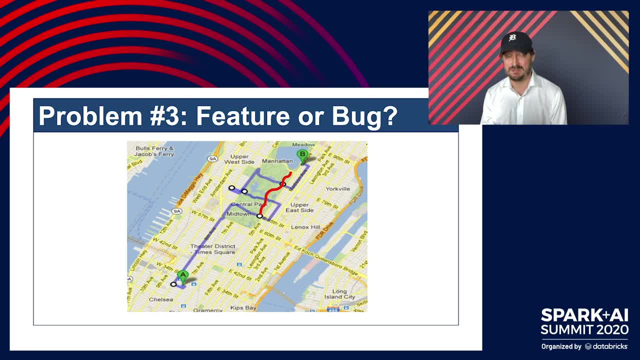 that you have right. If someone wants to sit down in a poker game and play you, they seem very eager to invite you to the game. You should maybe ask yourself: okay, Um, you know, am I the sucker here? potentially, Um and again, I'm not someone who says that markets are always right, I think. 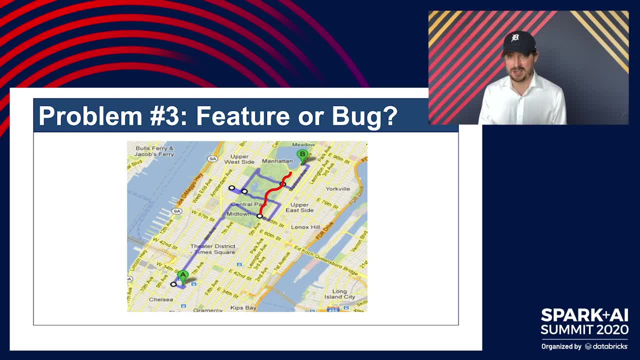 it's a lot more complicated than that. I think we didn't have people who tried to beat markets, and the markets actually wouldn't be any good Um. but a competitive environment, um is a lot different than one in which we're the only person out there looking for intelligence and for signals. 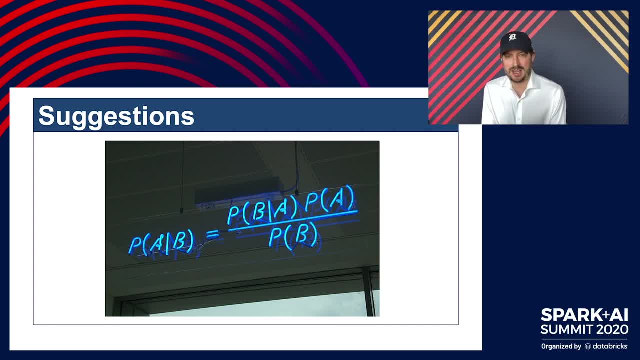 Okay, So I want to move now into the more, I guess, um optimistic part of this: to start to suggest some, um, some heuristics for how we can go about doing better analysis. Um, and none of these are terribly technical, right? You see here a sign depicting Bayes'. 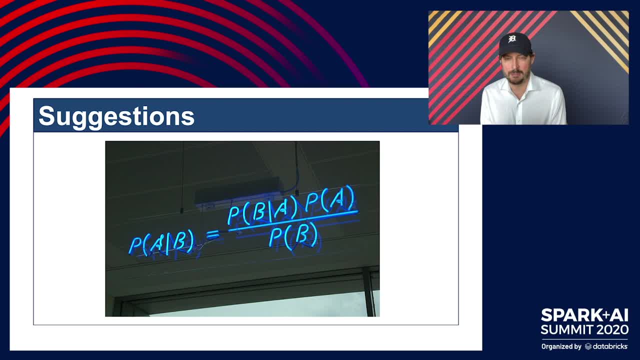 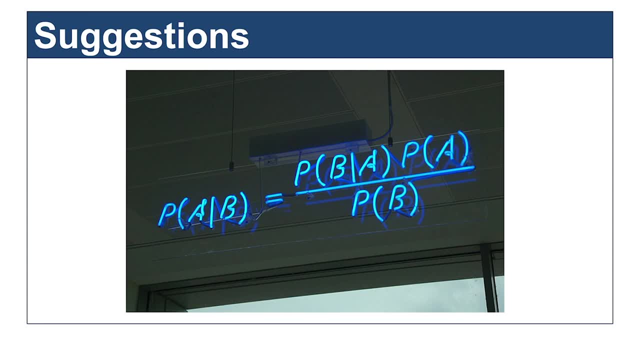 theorem that I'm sure a lot of you are familiar with, The Bayes' theorem- is a um, a very um old algebraic formula that just tells you how to weigh new information and how much to update your beliefs, given what you know already. Um, you know if you are in a meeting. 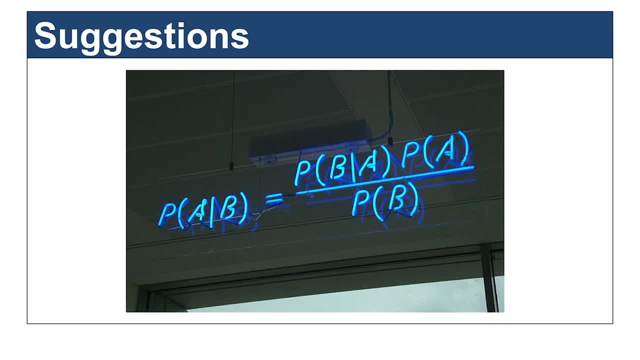 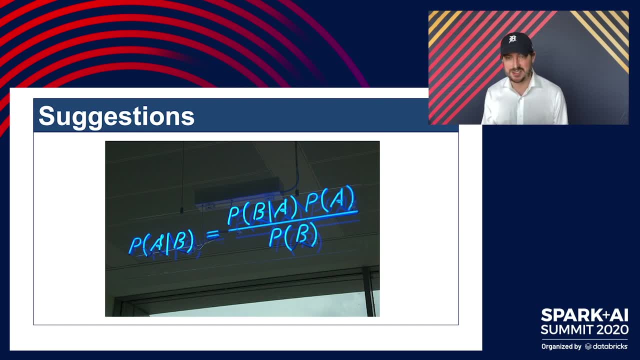 you probably are familiar with the concept where you kind of walk in and you're very- um, maybe you're zooming now, right, You don't really know very many people, You're very naive and you kind of refine your views as you get more information, in some ways to very intuitive. 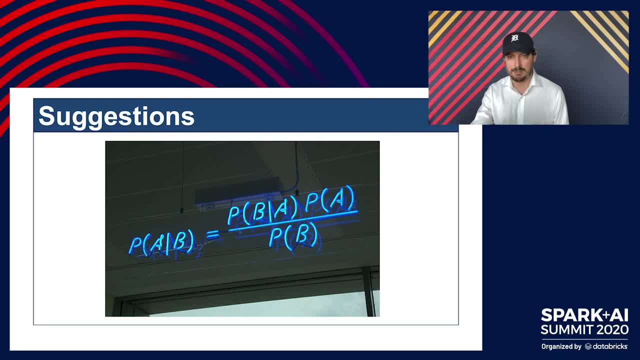 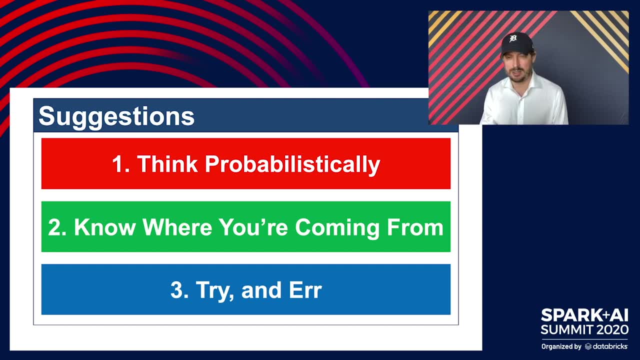 process, But it does involve some things that, um that are are important to keep in mind when, when, we're doing analysis. Um, so three things, and these all kind of stem from Bayes' theorem. Idea number one: think probabilistically. 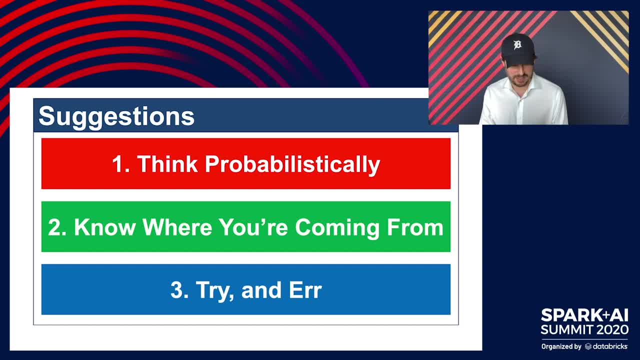 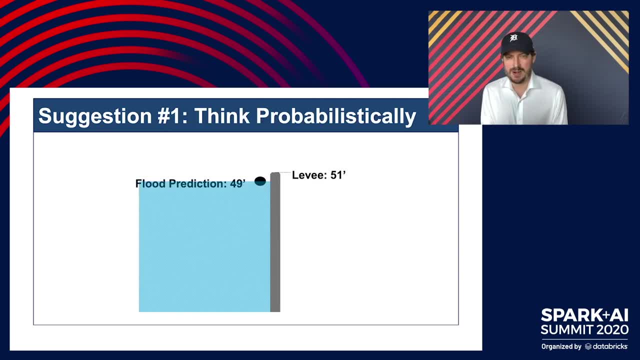 Idea number two: know where you're coming from. And idea number three is try and error. So I'm going to explain each one of these in a little bit of detail here. So if you know anything about about FiveThirtyEight um, or know anything about 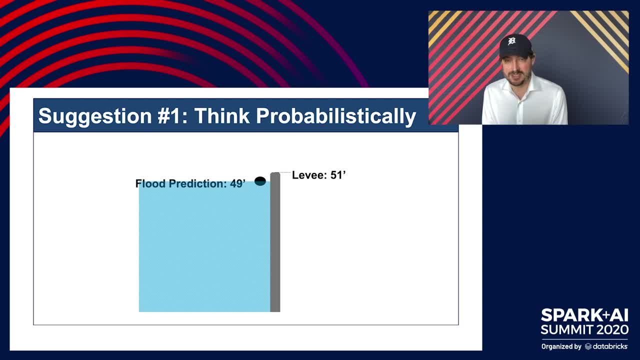 my work then. um, we are kind of obsessed with probabilistic um forecasts instead of deterministic ones, right? So, whether it's Trump having a 29% chance of winning or, um, I don't know, the Toronto Raptors having a 51% chance to win the NBA finals or something against the. 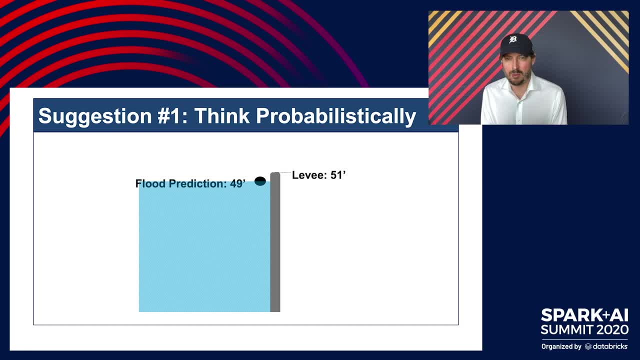 Warriors, um, last year. um, you know, we've always kind of been obsessed with, um, trying to measure uncertainty and add value in that way, Um, and there's a reason for that, which is that, um, there's a long history of people being poor about communicating uncertainty and actually, 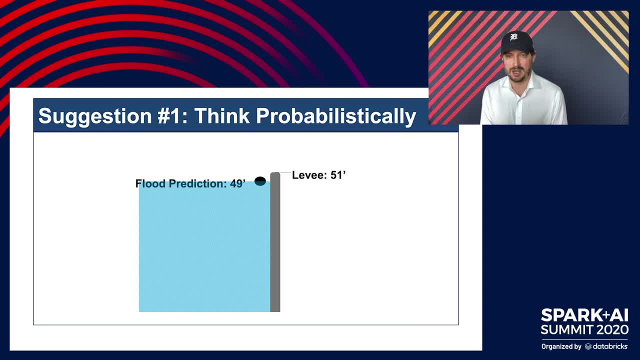 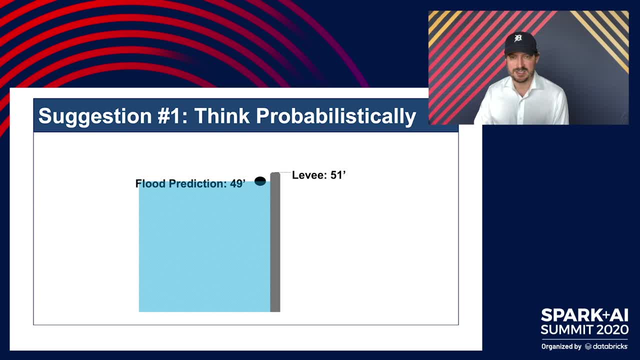 the red river of the north, and what happens there is that um is that there's a lot of snow, obviously up in north dakota. so, roughly speaking, every march that snow begins to melt and if that snow melts pretty fast, you have the risk of flooding in the rivers in north dakota. um. so one year in 1997, 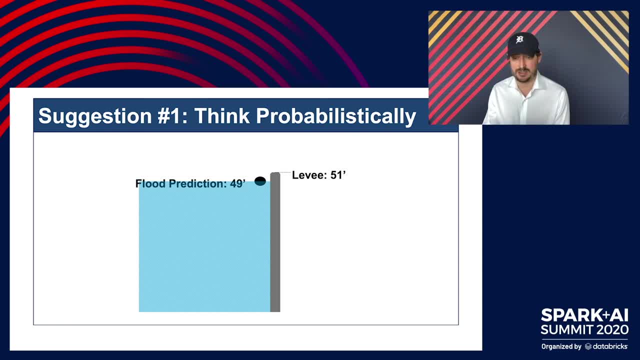 there was a particularly large risk of flooding. one service issued a forecast saying: hey look, we have done the math. um, this is not like hurricane katrina. this flood is happening or the water is melting slowly, but but predictably and kind of inevitably, but say we've done the 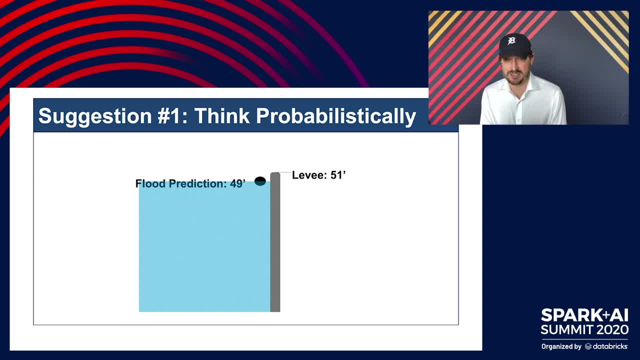 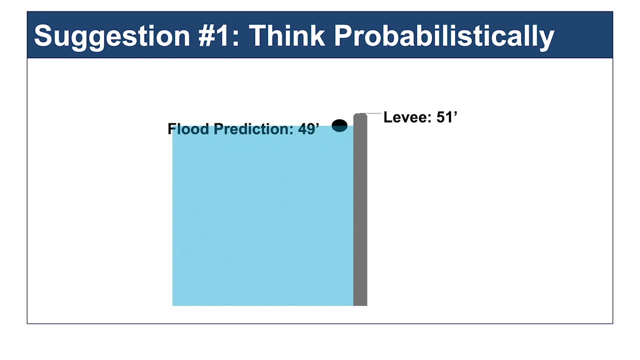 math and look on the worst day, we think the flood, flood waters were pressed at 49 feet. um, so people in grand forks, north dakota, said, okay, well, that's okay. 49 feet is a little scary, but we have flood walls that go up to 51 feet, and so we can do the math here: 51 is greater than 49. 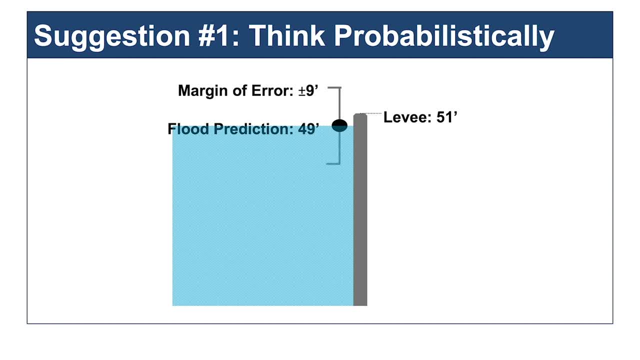 so what's the big problem? right, well, the big problem was was this: that the margin of error on the forecast made weeks in advance was plus or minus nine feet. so in fact it was almost a 35 or 40 chance the levees would be toppled by the water. in fact, that's of course. 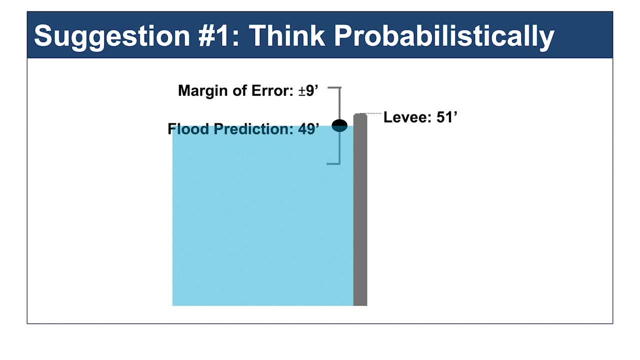 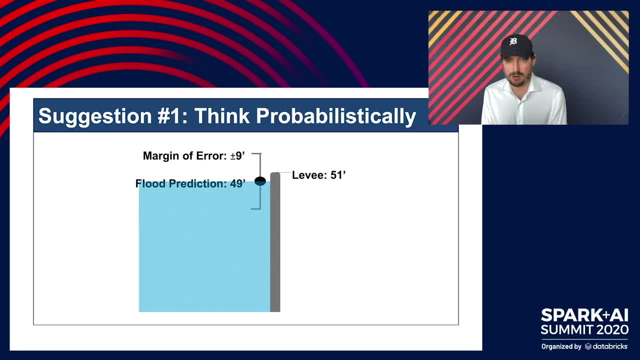 what happened. the water's actually pressed it at 53 feet on the worst day of the flood, so you're actually well within the margin of error. um, it's a good forecast in that sense, but it's a binary outcome where all of a sudden now, um, almost all the town is flooded. people did get out with their 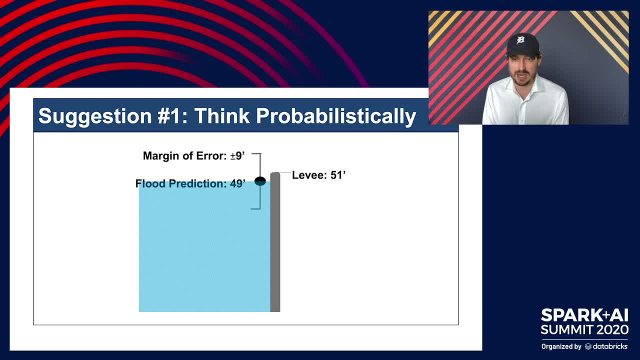 lives on a loss of lot, not a lot, not a lot of loss of life, but you did have um fairly severe flooding and a lot of uninsured property dams that could have been avoided. people had actually looked at the margin of error. um, the problem was that the weather service really de-emphasized the margin of 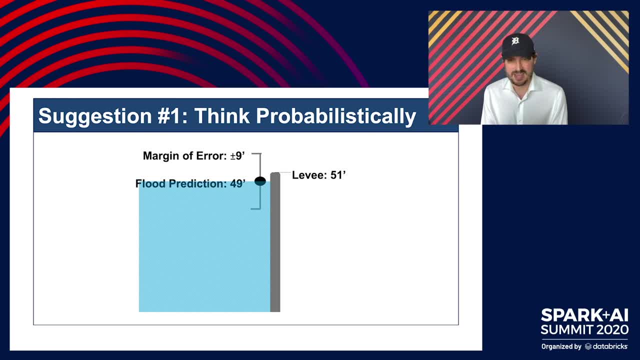 error in their communications about the flood. um, they were afraid that if you convey uncertainty, that people think that, hey, you don't know what you're doing. i think we need to really reverse that perception all the time in society. right um to me, if i am evaluating, say, a job candidate, 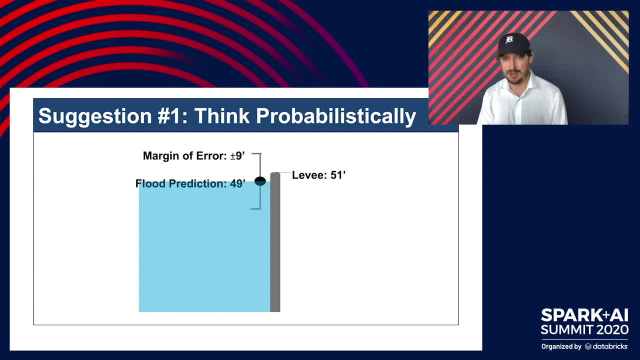 at 538 and they come in with a model and they say: hey look, i can predict with 100 accuracy who's the next election. i would tell them politely to get out right, because you can't have a model that is that accurate. um, that means you've done something wrong. probably overfit would be one. 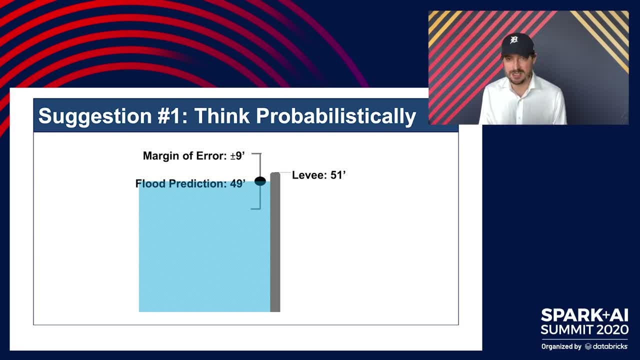 way to do it or kind of p hack your way um minimize uncertainty. instead, we want to measure this and quantify this and try to calibrate it so that when we actually say there's a 30 chance, it actually does happen about 30 percent of the time and not more or not less. um and again, when it comes to covid, 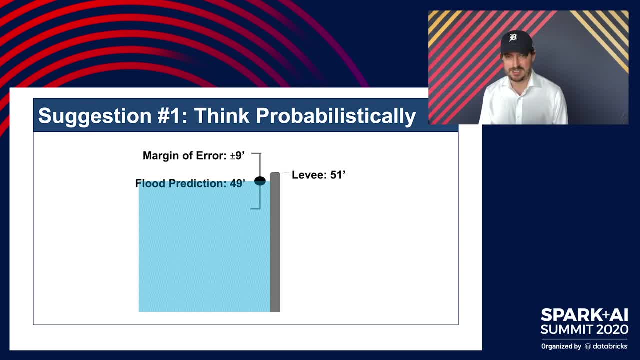 um, you'll sometimes see kind of public health agencies talk about uncertainty in really odd ways, right um, with masks, for example, where most of the evidence kind of now points toward masks potentially being very helpful to wear, where, well, at first, the who and cdc, the place we're like- well, it's not proven that masks work. therefore, maybe you 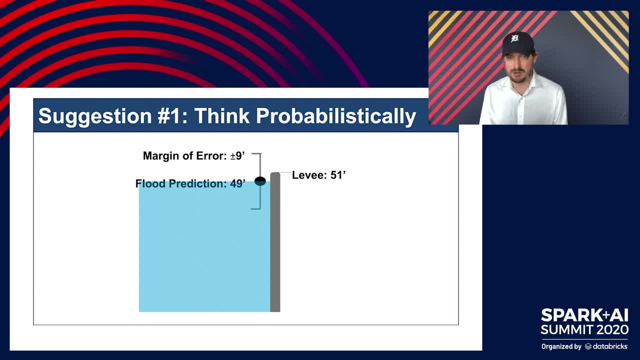 shouldn't wear them right. well, you know that's actually not very helpful if you're trying to deal with problems in real time. um, then having the near preponderance of evidence saying, hey, we think masks probably work. it might not be proven, but like, actually it's probably still. 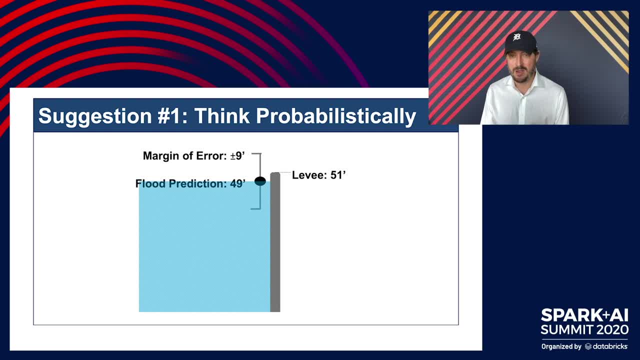 going to be a very effective way to kind of make it a relatively low cost way to prevent and lower the risk of spread? um would have been having everyone kind of wear masks, not just starting in april and may but back in march. it might have been a lot better that way, frankly. um, so you know. 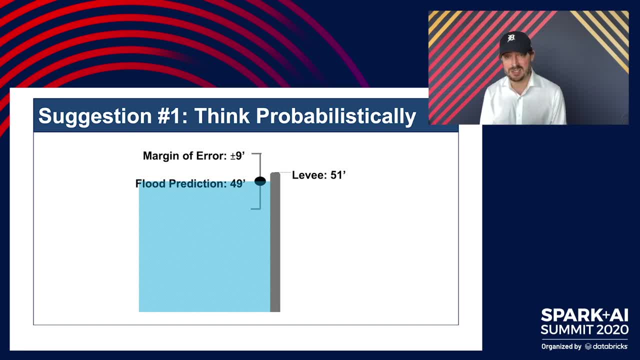 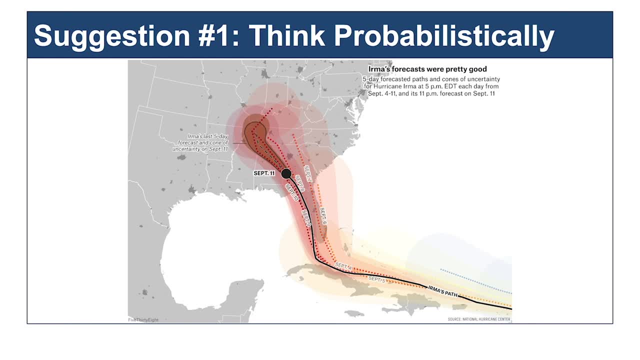 encourage people to to include probability, to include complexity in their explanations and not kind of shutting them down when it seems like they have a more nuanced answer. i think is really, really important. um, by the way, i don't mean to make um too much fun of weather forecasters. in fact, if you 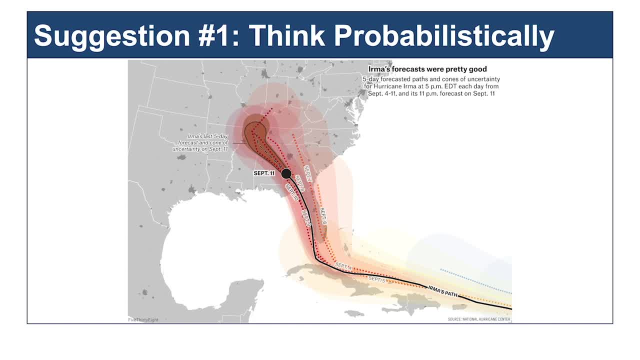 read um the book. weather forecasts have gotten an awful lot better over the course of the past uh, 30 or 40 years. um, you see, for example, how accurate the forecast was for hurricane irma when it hit florida a couple of years ago. and yeah, but the track shifts a little bit. people sometimes think it's. 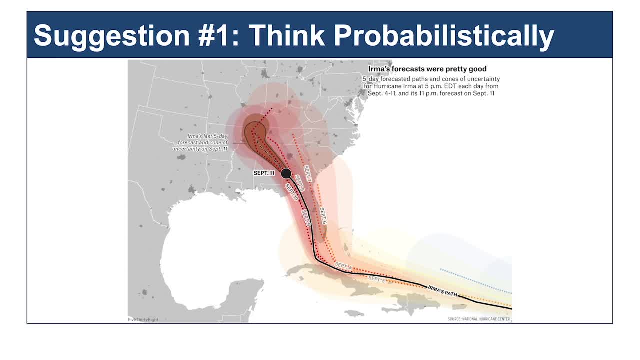 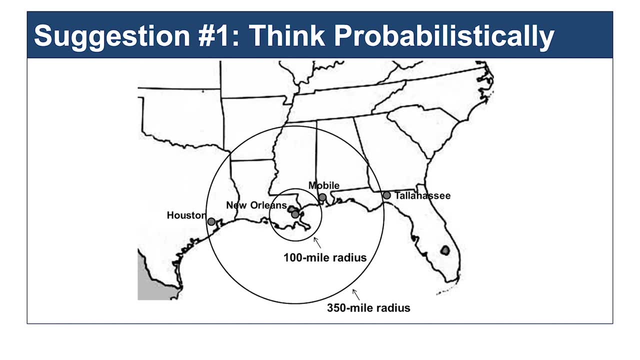 overly precise in terms of the exact county or city, but basically these things are improving a lot. um so, for example, about 30 years ago, if you had a hurricane in the gulf of mexico, on average there was about a 350 mile error between the forecast and where that and what. 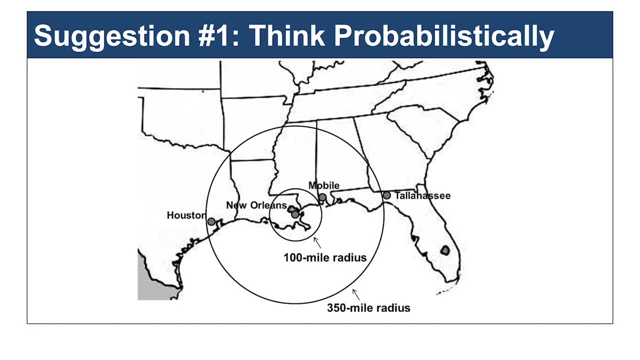 that hurricane actually hit. so three days in advance you might have a hurricane in the gulf of mexico. it would hit anywhere between half the time between houston and tallahassee, florida, roughly. the other half would be somewhere. somewhere else entirely would hit mexico or curl up and hit. 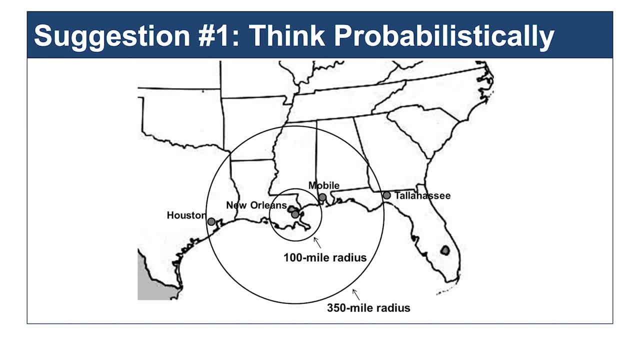 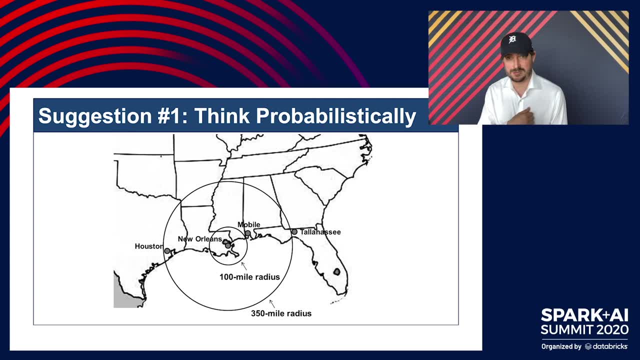 north carolina, um, or whatever else. right, it's like not very useful and actionable intelligence. um, nowadays, forecasts are within about 100 miles, on average three days in advance. you can see on the map that a 100 mile radius is actually very actionable, where you can evaluate, where you can. 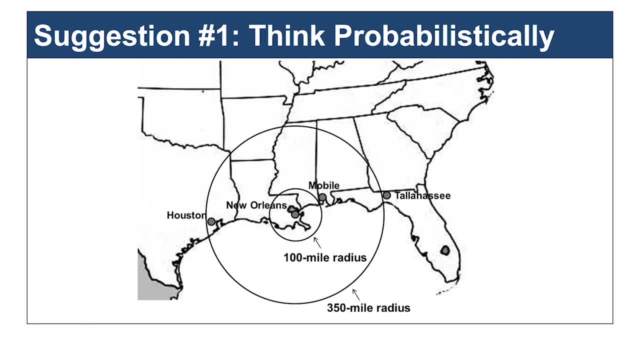 evacuate on the jersey shore or evacuate houston or new orleans or a place like that. and although we have not found a way to stop hurricanes or prevent property damage, there is much less loss of life now from most hurricanes because we have a better forecast and more advanced warning, and 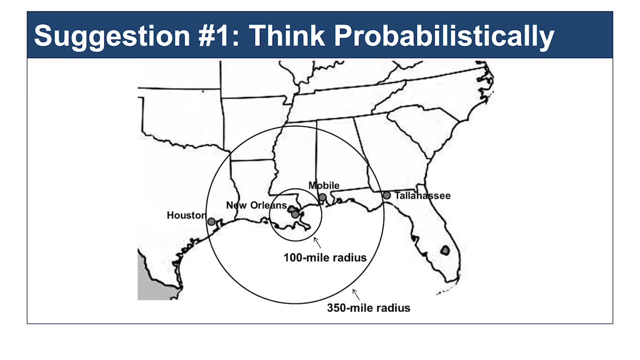 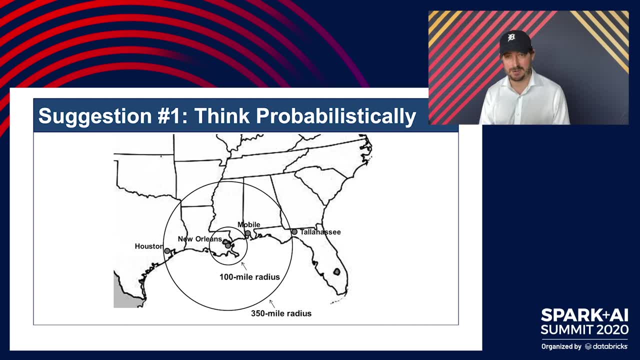 that has led to leaps and bounds with an improvement in terms of saving people's lives from the storm. by the way, before we go too much further, i want to stipulate: i am not going to talk in these prepared remarks about the 2020 election. i'm going to save that instead for the 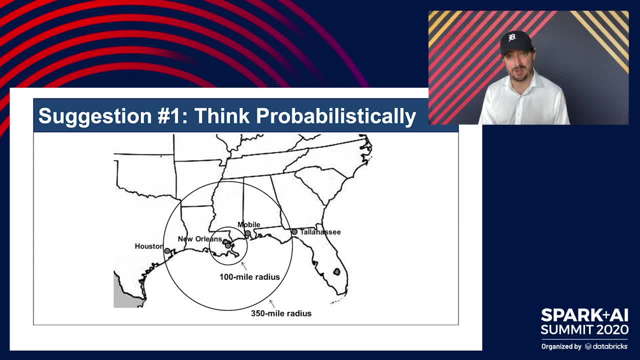 um, where i'm happy to take questions. that's for a lot of reasons. maybe first and foremost is that we do not officially have our model ready yet, so we have no kind of authoritative take on the election yet. but of course i have lots of insights. i have been working on the model, so i 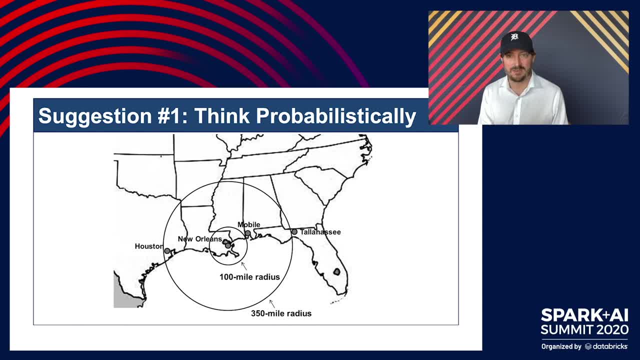 have some clues about what it might say. um, of course, a very momentous election, um, but i want to kind of save the election, talk for more of an interactive format and focus more on some of the kind of abstract principles and examples from other parts of the news and other parts of my life. 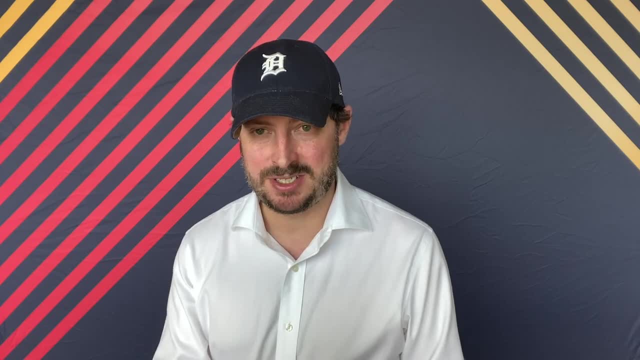 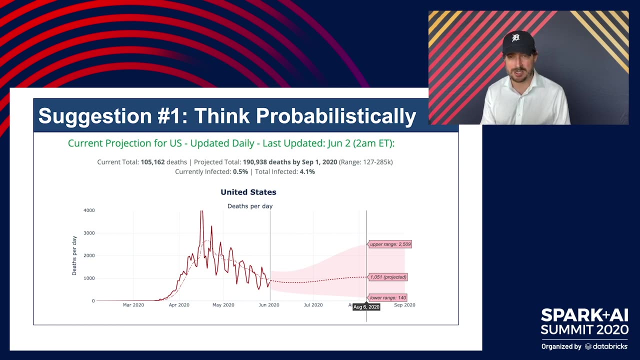 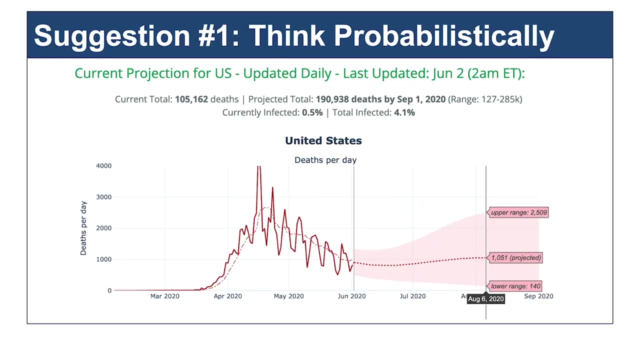 here. uncertainty, of course, is also very important when it comes to looking at infectious disease, for example, where this is a forecast from of coronavirus, from a guy who actually um who actually formerly was a hockey analytics guy at mit- um he has what is so far the best coronavirus. 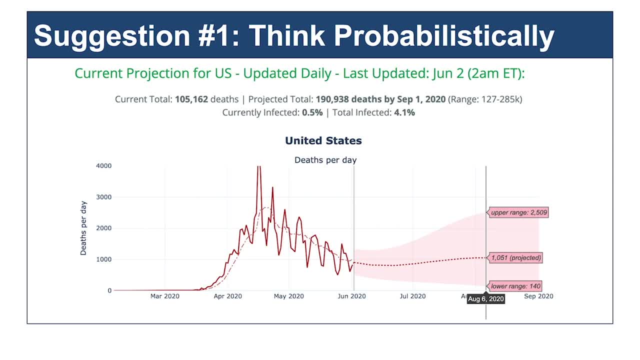 model used machine learning. it's very sophisticated and smart, um, but it's another example where actually his model has really wide confidence bands. if you project out, for example, until august have as many as 2,500 people a day, or as few as 140 people a day, dying per day from coronavirus. 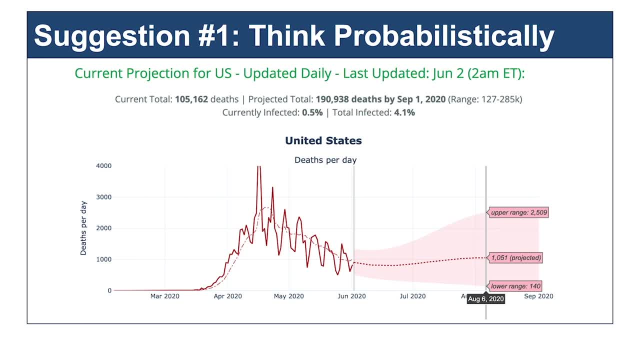 It's been about a thousand, for example, in late May and early June. So you know, people can get frustrated and say: well, you're trying to give like you know, you're trying to give such a wide range, You're kind of covering your ass, right. Well, the fact is that experience tells us that 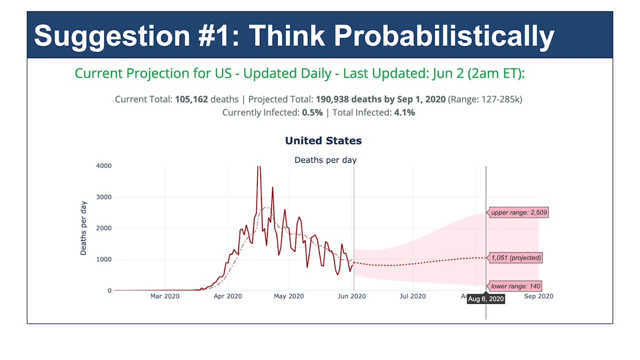 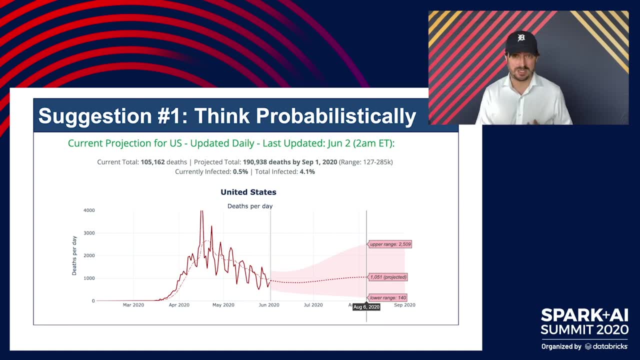 that's actually about as well as people can do, Given. we don't know very much about people's behavior. we don't know that much about the disease itself. We don't know, for example, how much will transmission be lowered in the summer. We're just learning more about how. 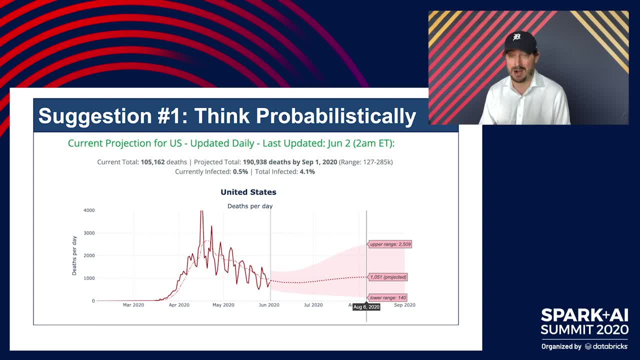 for example, protests might spread coronavirus, how Memorial Day barbecues might. whatever else people have been doing in May and June, That stuff makes it kind of hard to forecast And again, there is no prize to be won from false certainty. You may feel good about it at the time It may. 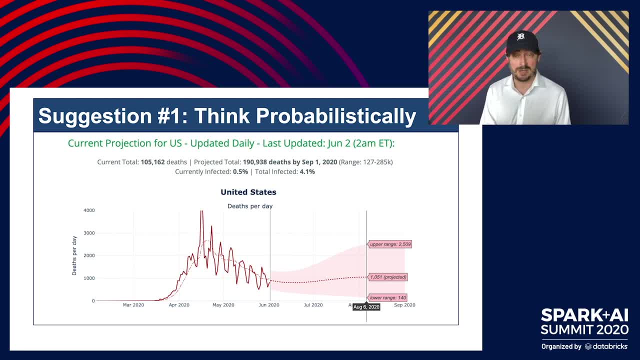 make it easier to pitch on TV or something but like. but we know from many years of experience that being able to build accurate confidence, you know, and account for uncertainty is kind of where the actual skill comes in. So if you look for a COVID, 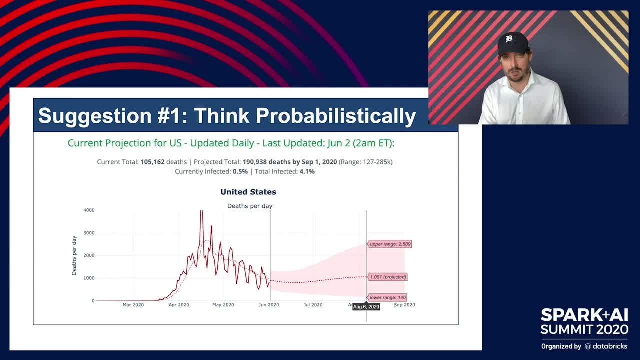 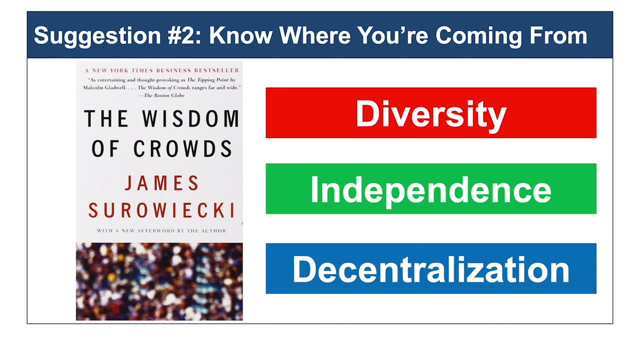 projection. the wider those ranges are, the more the person probably actually knows what he or she is doing. Idea number two is what I call know where you're coming from. So it means being aware that we each have a subjective point of view. again, does not mean that there is no objective. 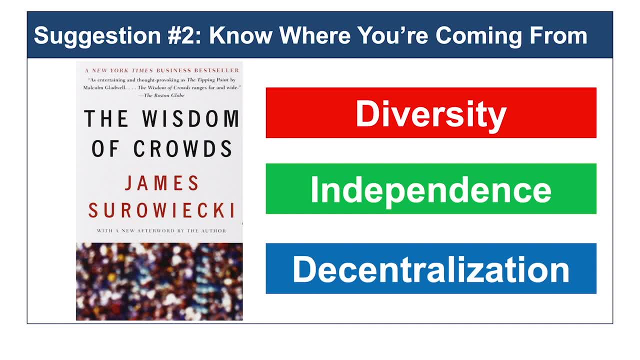 world, but we're all trying to grope at it with our own kind of jaded perspective. And so what are things you can do as a person or as an organization, maybe more importantly, to give yourself a better chance of actually perceiving what the objective world? 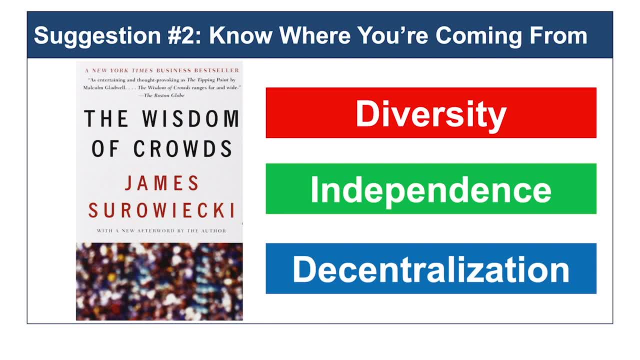 actually is. Well, I would recommend, in addition to my book, reading James Surowiecki's book The Wisdom of Crowds. He is an editor, a writer at the New Yorker, And he talks about what characteristics tend to make crowds or groups wise, versus what things make them dumb can lead. 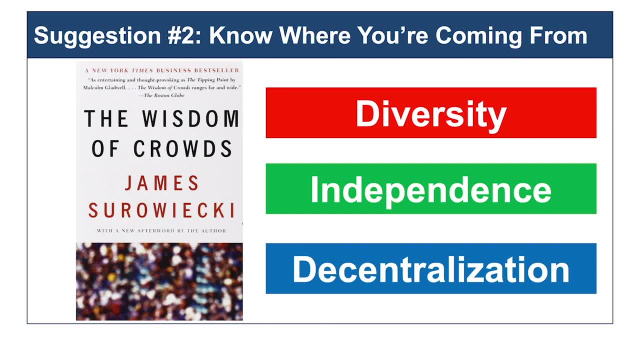 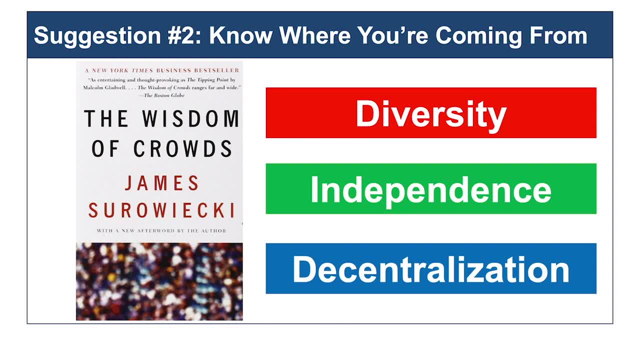 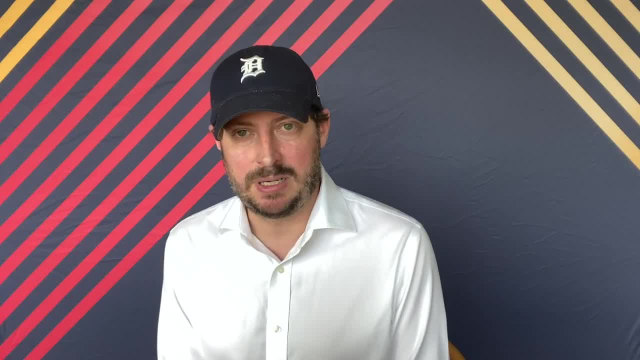 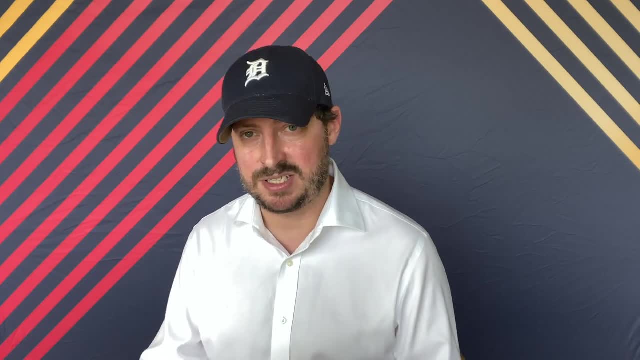 having people from different ethnic and racial backgrounds and different genders and different income classes and whatever else from parts of the country or the world. I think that definitely helps and is important. But diversity also means, often related to that, having different modes of thought, different skill sets, different strengths and weaknesses, different tolerances for risk. 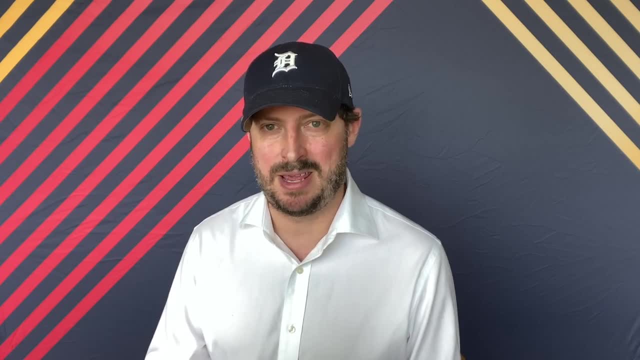 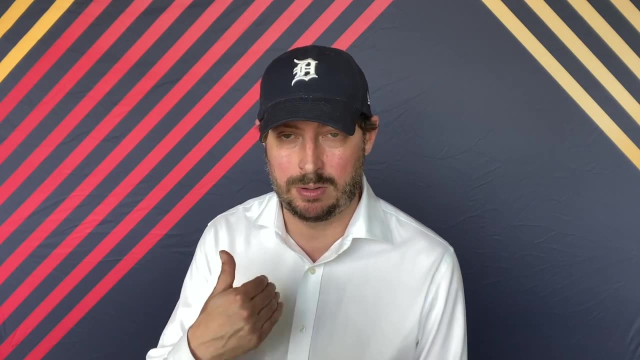 or whatever else. Look, if you take a hundred smart people and put them in a room together, they may be brilliant, But if they all are smart in the same ways, then you may as well have just one person right? So the whole. 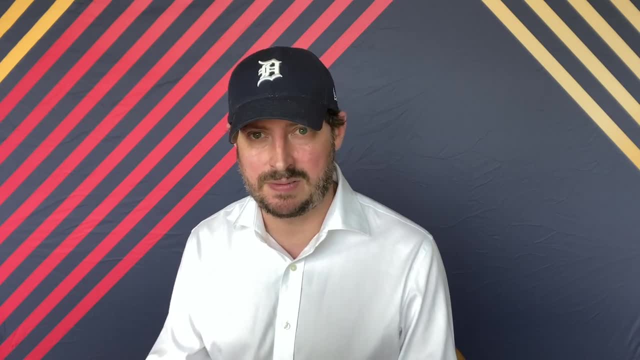 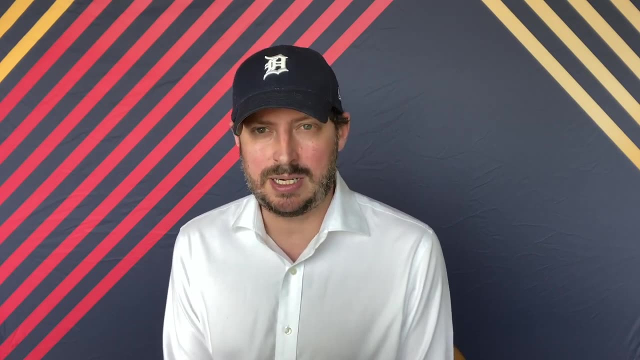 notion of having a diverse crowd is having different skill sets of perspective that are brought to bear and try to piece out what the real world actually looks like. Number two is independence, where people have to be empowered to actually articulate their view of the evidence. 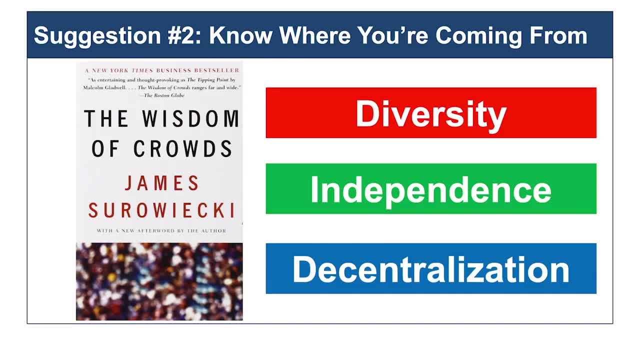 If people are not empowered through that, then you are going to have groupthink over almost first year. So if you're not empowered through that, then you are going to have groupthink over sure. So having organizations where you're allowed to question your boss- right, You know. 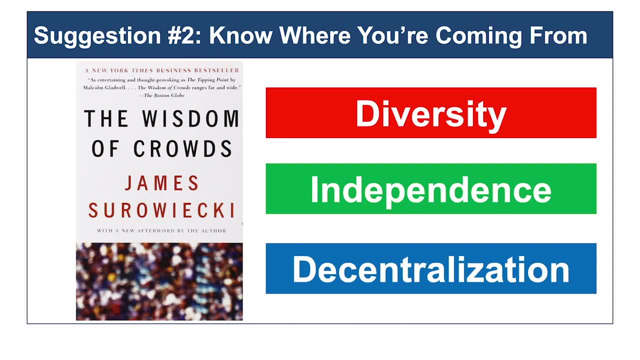 I kind of am people's boss now at 538, and one thing that's actually pretty hard is to make sure that people are able to give you feedback and aren't fearful of the results and consequences of that right. I think I'm pretty good at that, but it can be intimidating sometimes to people. 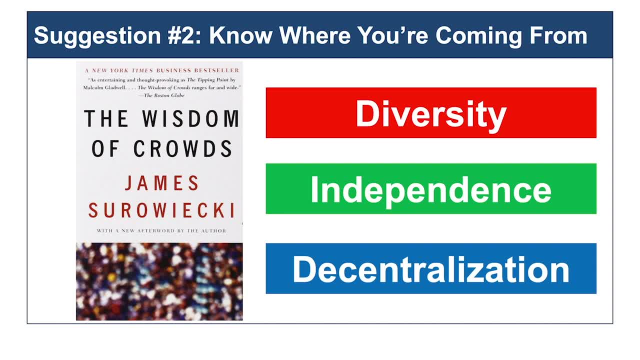 Making sure in governments, for example, that people aren't all trying to impress the governor or the mayor or the president, For example, and having groupthink that way. So having real incentives for independent thinking is important. And the third characteristic is decentralization. So if people can really pick, 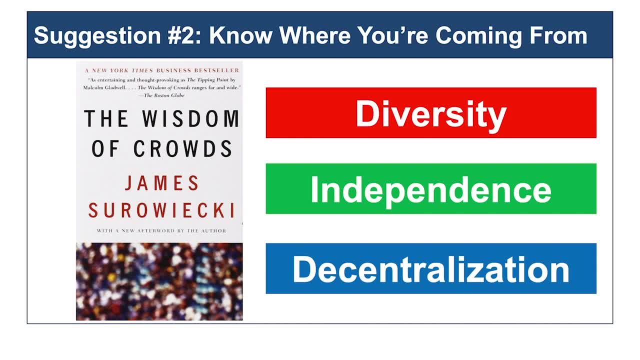 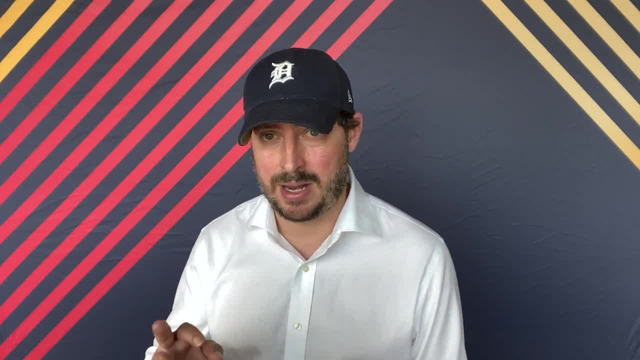 up local information and knowledge on the ground in some ways is very much related to diversity. That seems to help a lot too. If you can actually add net information to the problem, not just kind of regurgitate the same data, then that can add value as well. 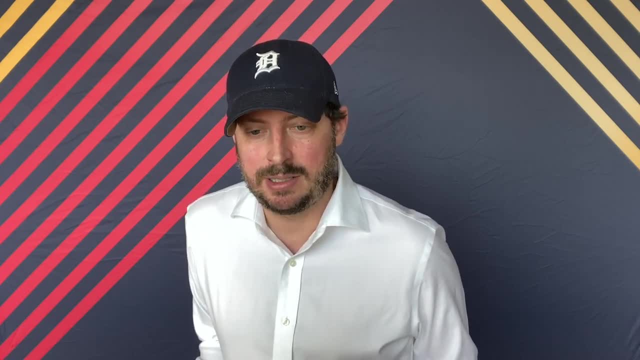 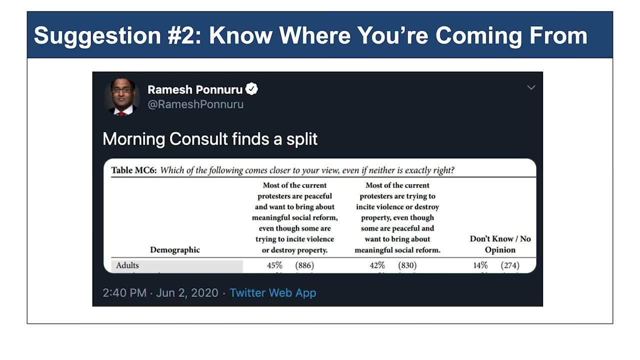 Of course, when we're in very polarized times politically, then people can take very different views of the same underlying facts right So, right now, for example, if you look at- okay, what were views initially of the protests as they were unfolding? 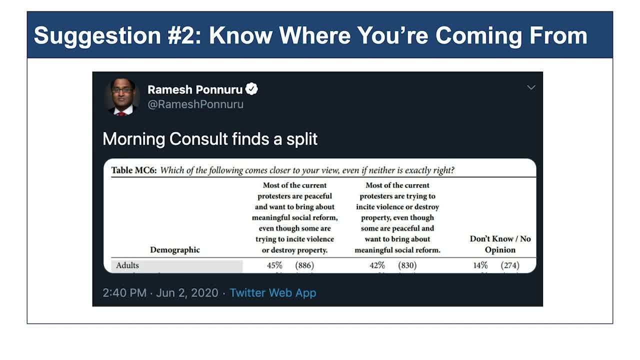 in early June. it was literally almost 50% of people who saw them as protests, primarily, on the one hand, people who saw them as violent, even riots on either hand. Again, it's not a surprise if you follow American politics, that polarization. 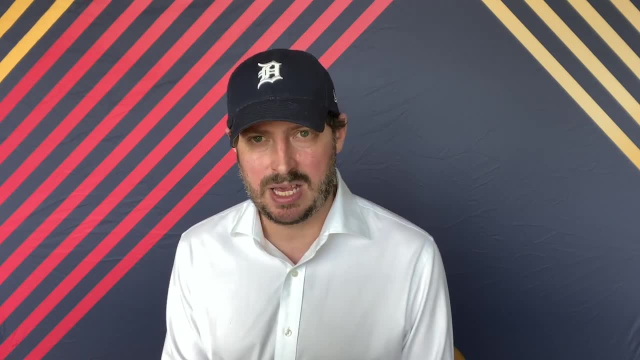 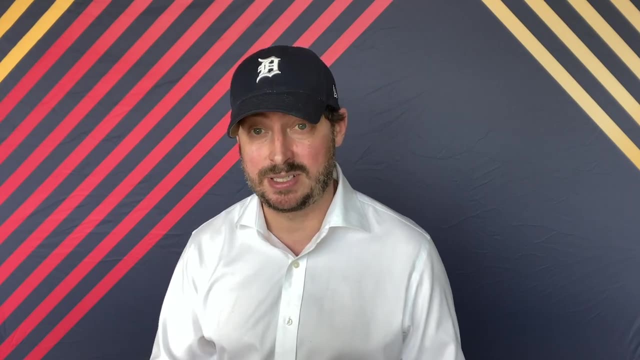 is increasing. But I think it's important to be able to keep in mind that when you are looking at something from your point of view- and we're now on social media all the time- we're now in environments where we're able to easily kind of share our points of view and able to kind of 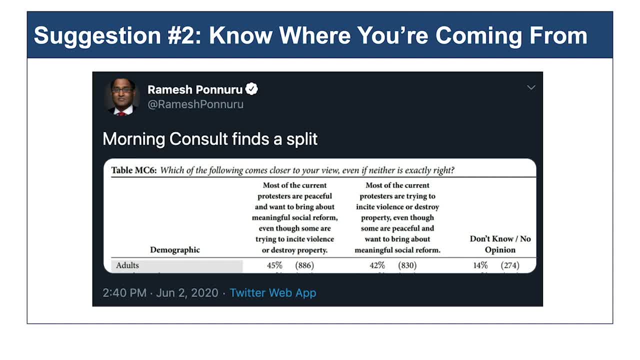 filter together what we consume in the media, that we read and get affirmation or confrontation, whatever else. that way it's pretty important not to get in what you might call a filter bubble where we only kind of see things that tell us a certain side of the story. And so I think 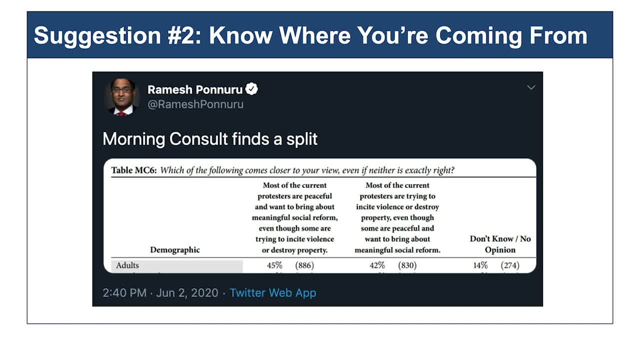 if you look at the Democratic primary, for example, when Joe Biden won, that surprised a lot of people, even though, especially on Twitter, on social media, even though Biden had been ahead in the polls for all of last year, he did fall behind after Iowa. 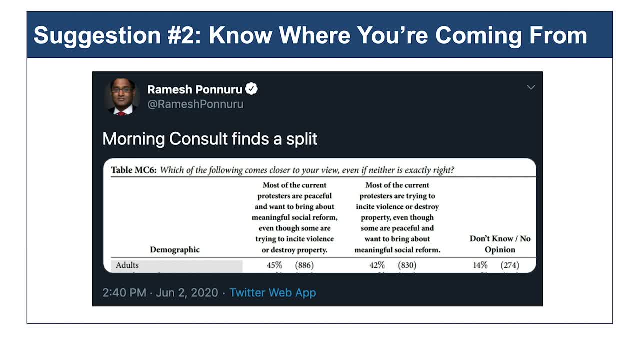 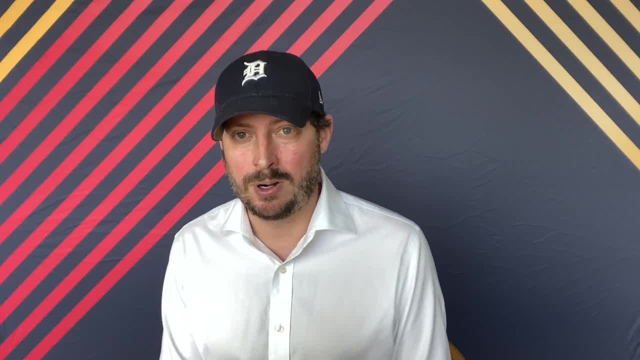 and New Hampshire and Nevada, but he had been one of the front runners all year long. It was not a huge shock that he won, but you don't encounter very many Biden supporters online that tend to be older and poorer, less digitally savvy, at least in the primary, And so people need to. 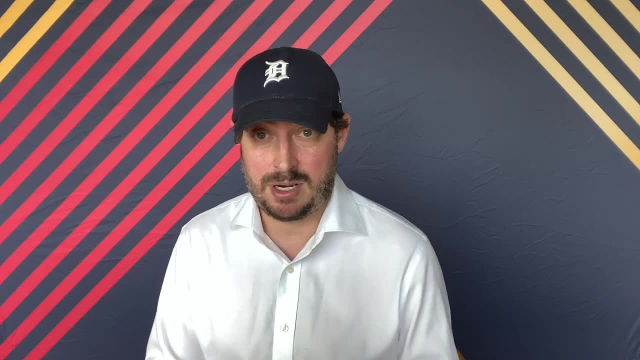 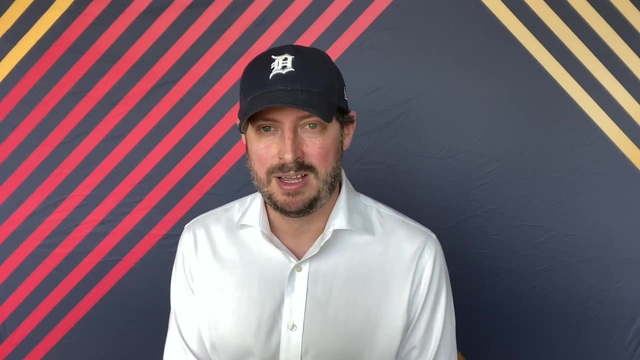 understand that what you might experience in your peer group- I'm not saying your peer group is wrong- right, You probably pick them carefully. you believe in their values. you maybe like their values. they probably have good values. right, But still being able to look at the world from. 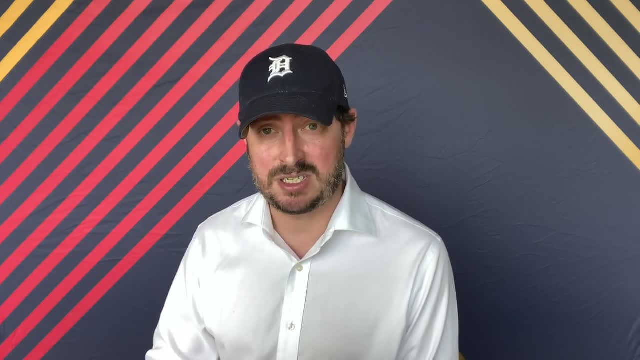 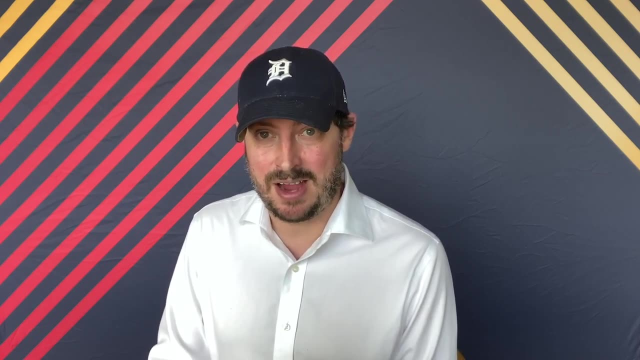 different perspectives and being able to say: okay, look, I understand that I might be a smart person, but I have certain biases and certain beliefs and certain priors. So you have to kind of actually listen when someone approaches the world in a different way and not just assume that. 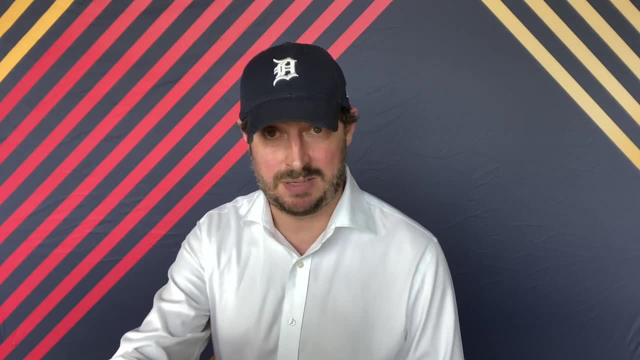 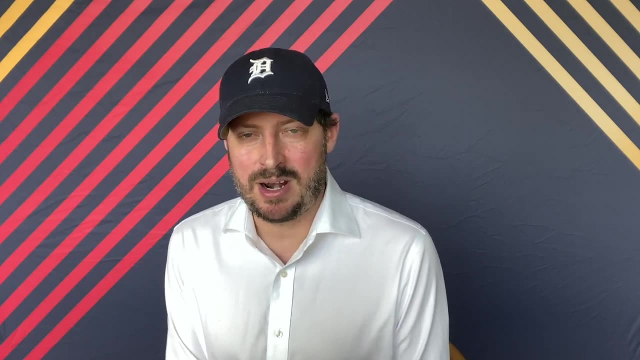 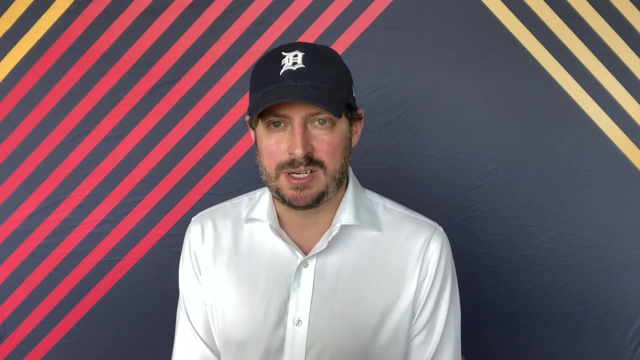 misinformed or evil or corrupt or whatever else. Sometimes they are right, But not a good default assumption. The last thing here. I want to finally focus on a few more lighthearted examples before we get back to talking about politics and so forth in the Q&A. But trial and error is really 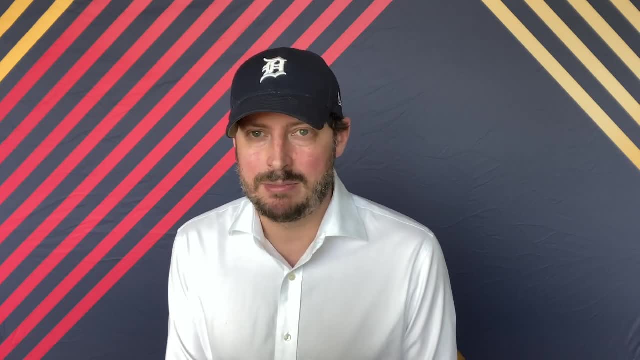 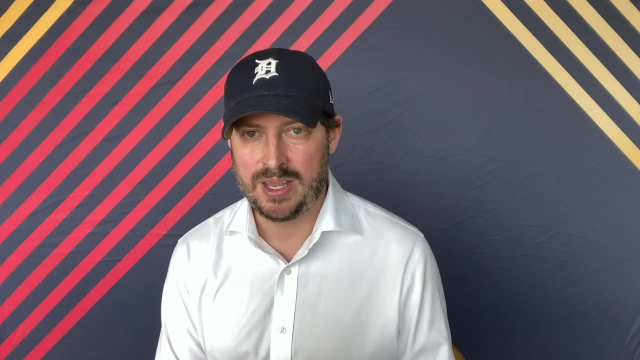 important. Having spent a lot of time now building models, releasing them to the public, I know that very often you can whiteboard things, you can scenario plan as much as you want, Until you actually have a product tested by actual users, by actual people. then 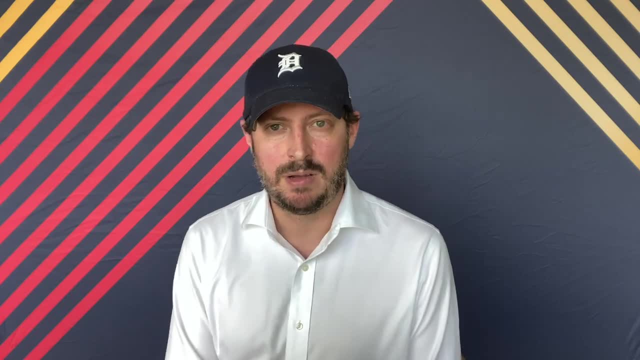 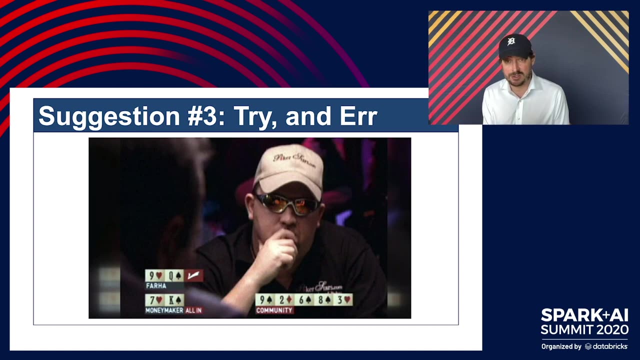 you can be very surprised. I'll take an example here from poker instead. So way back in the day I had a job my first time out of college as being a transfer pricing consultant. I will not get into the details of what transfer pricing is, but it's roughly speaking. 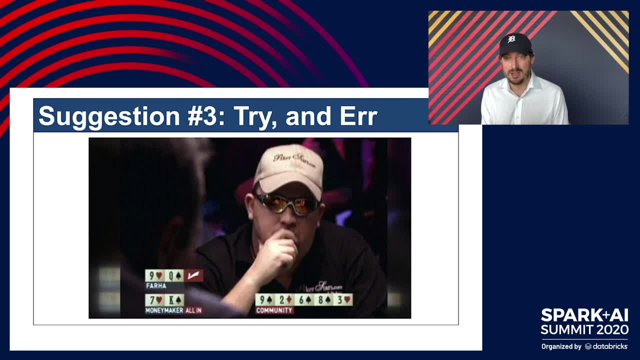 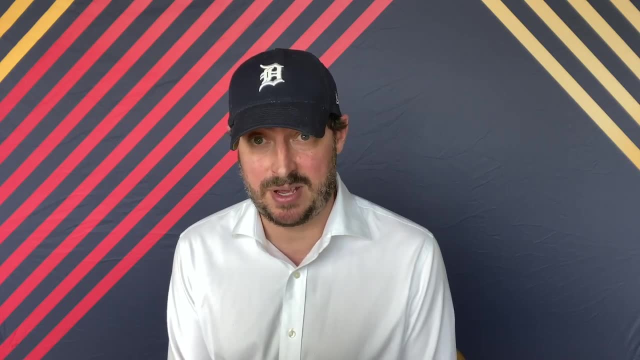 as boring as it sounds, This came at a time when there was something called the poker boom around the country where, because of ESPN and hands like this one that you see depicted here, poker is becoming a very big thing in the United States. This is a hand from a screencap from ESPN. 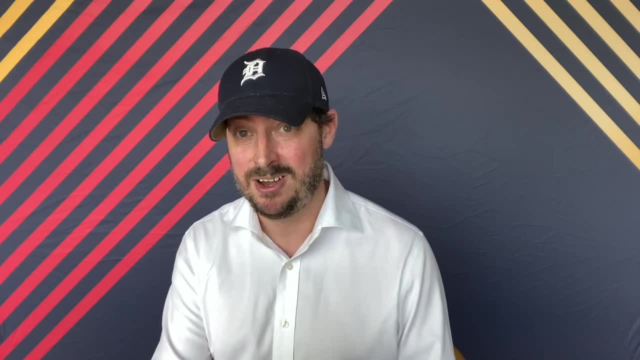 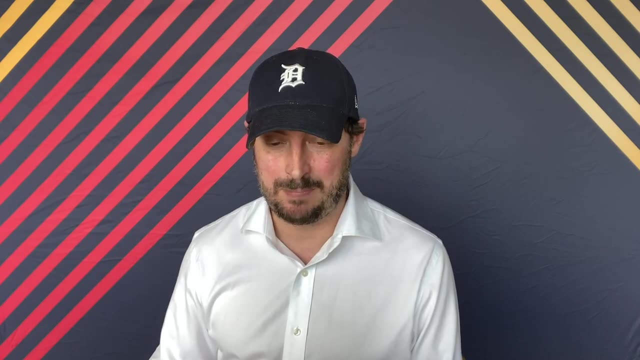 where Chris Moneymaker, who actually played Chris Moneymaker recently in a charity poker tournament. he is actually a very smart and skilled player and a nice guy, But this is a hand where he is bluffing against Sam Farha, this old kind of grizzled pro. 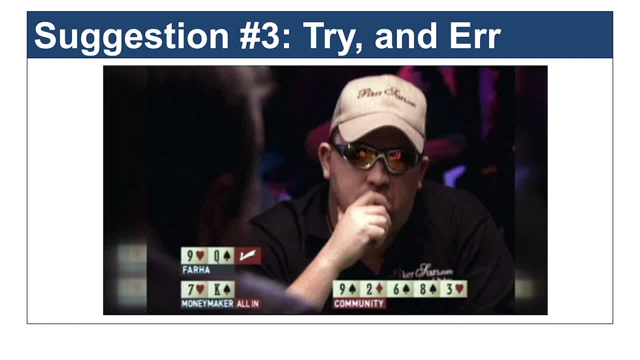 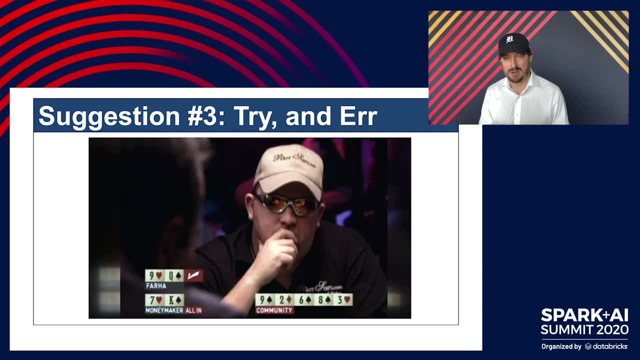 Chris Moneymaker's draw and miss. he goes all in. Sam Farha folds and Chris Moneymaker wins the pot. He wound up actually winning the World Series of Poker that year. So he went from having a job like mine as consultant, paid 20 bucks to enter an online qualifying tournament. 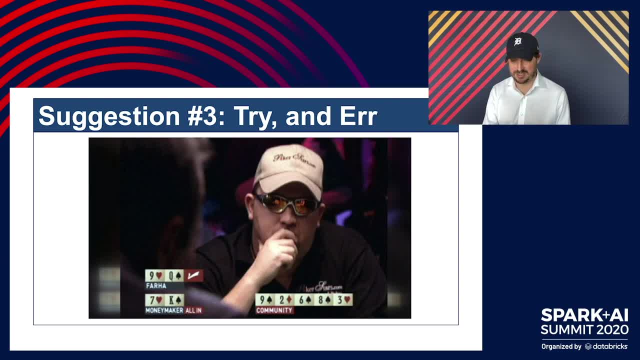 and wound up winning two million dollars first prize to the main event at the World Series of Poker. The thing about poker, though, is that it's usually not that easy. For one thing: unlike the slide you see here in the real world, you don't actually get to see what your. 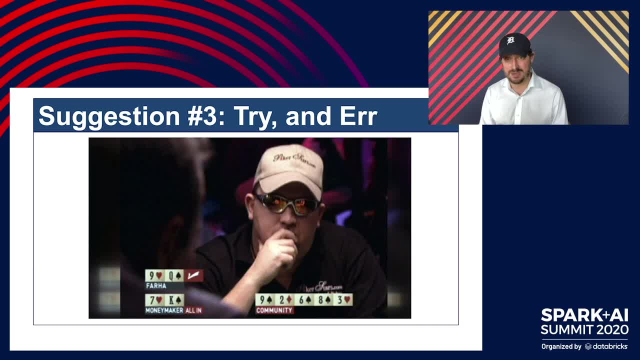 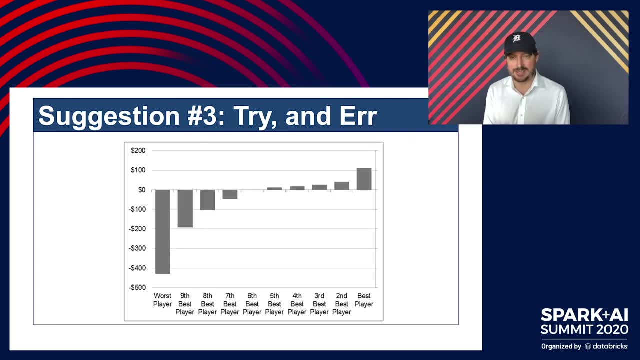 opponent's cards are until after the hand right, So you're watching on TV. it's as though you're clairvoyant Much harder in the real world when their cards are face down And in fact when I played poker, I actually collected a lot of data on how different people were faring at. 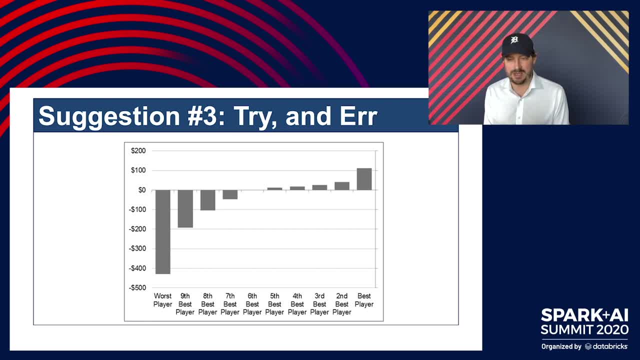 the poker table. First of all, no surprise, but most players are losing players and the worst players can lose a lot of money potentially. So, if you go- and this is data taken from a now defunct site- I believe it's still defunct. maybe it's resurrected in some form called Full Tilt Poker. 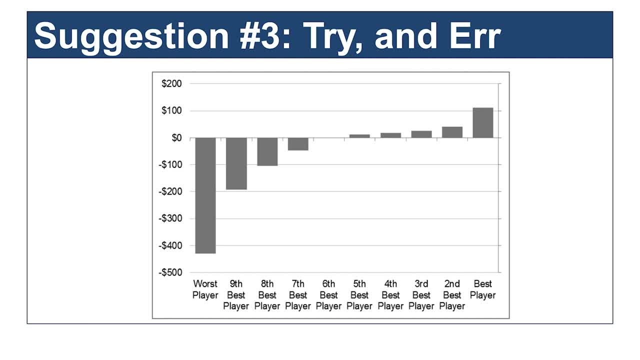 and looking at if you rank from the worst player to the best player at a 10 person table, how much money is each player making or losing over the long run? So it turns out that, first of all, it's way easier to lose a lot of money than to make money Where the worst player is losing more. 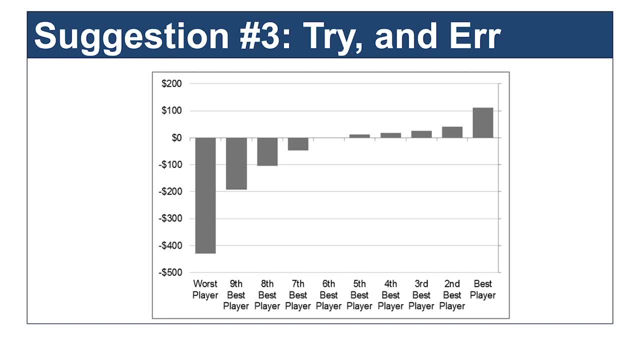 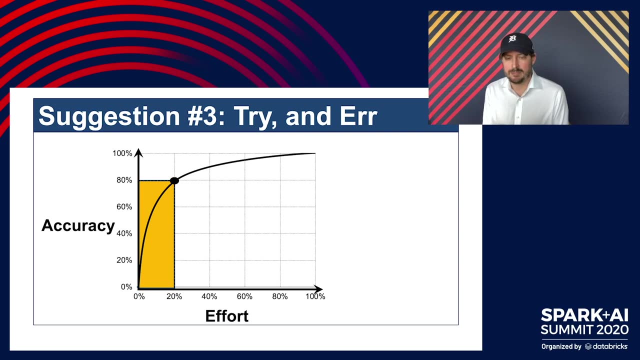 than 400 bucks per hour. the best player is only making 100 bucks per hour. Part of that is because the house takes a cut called a rake, and so the average person will lose money by definition, but still also reflects the learning curve when it comes to the complex data phenomenon. What 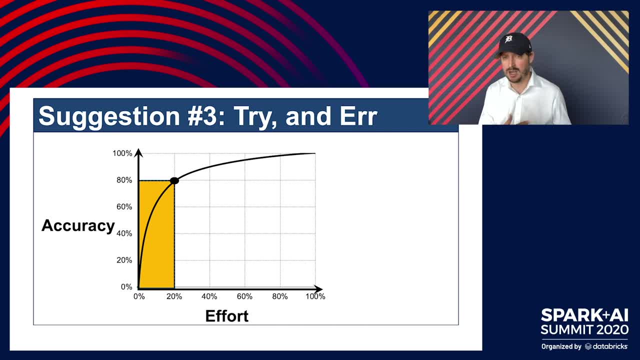 generally seems to be the case, though, is that there's a lot of data that's being collected and speaking. when you're trying to learn a new task, and especially when it comes to something involving analytics or when you're trying to build a model, then you gain a lot in the first initial. 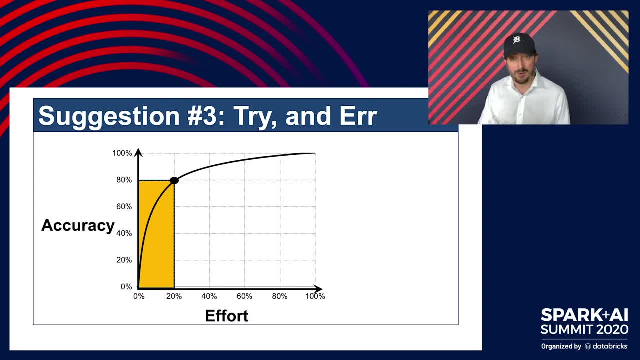 20% of effort. This is an 80-20 curve, which is, for example, in sales: you sell 80% of your price to 20% of your customers, and so forth. Again, this also applies to when you're building a model. 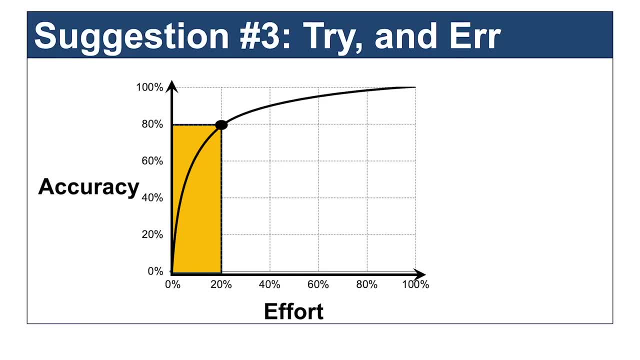 very often, for example, where, if you're looking at elections and accounting for major stuff like incumbency and how the economy is doing what the polls say, that will get you most of the way there and the rest of that is some more. 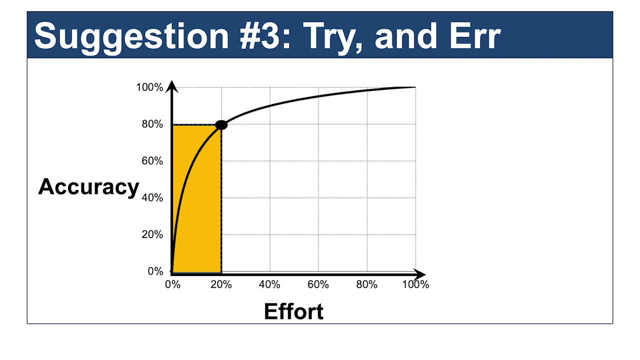 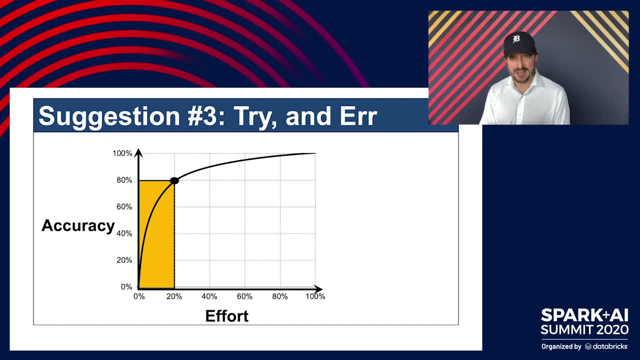 on top of that, If you're playing poker, then getting the basics right, saying okay, look, I'm going to fold my bad hands, call with my good hands and raise with my very good hands. that's the right play each and the time or so You have to bluff a little bit more. 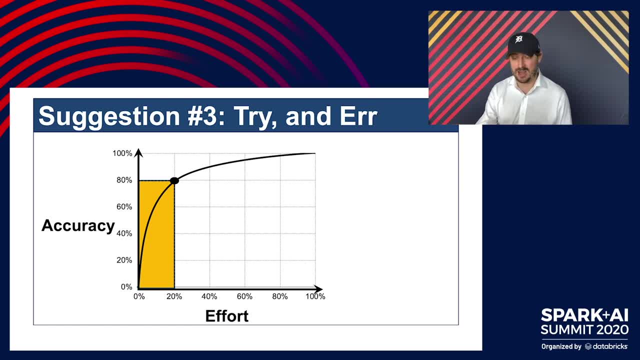 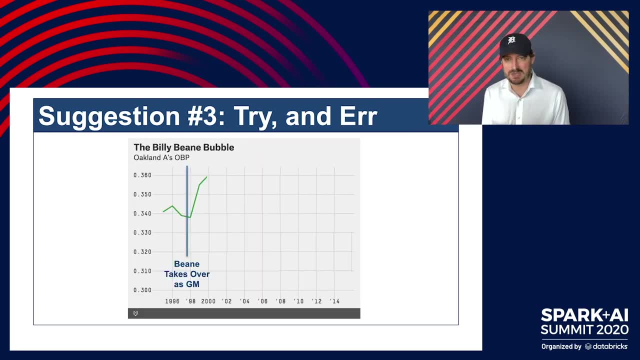 you have to slow play and trick people, but that's the more advanced stuff. You'll actually be a lot less bad by getting that first 20% right. One more example of this from baseball. if you guys have read the book or heard of the book, Moneyball, the story of Billy Bean and 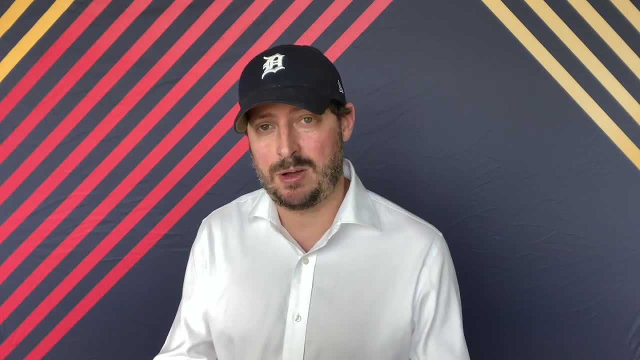 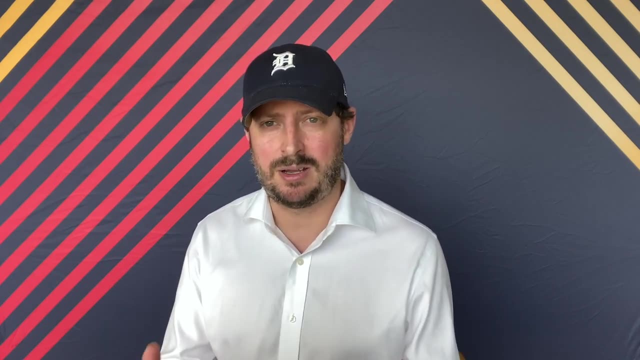 the Oakland A's. As Michael Lewis- great author, by the way- tells the story, Billy Bean takes over as GM of the Oakland A's. He understands that on-base percentage is undervalued in the baseball community. If you can get on base, you can draw walks. you can get hit by pitches, for example. 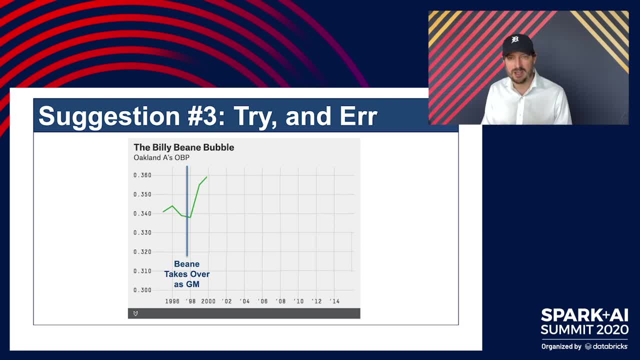 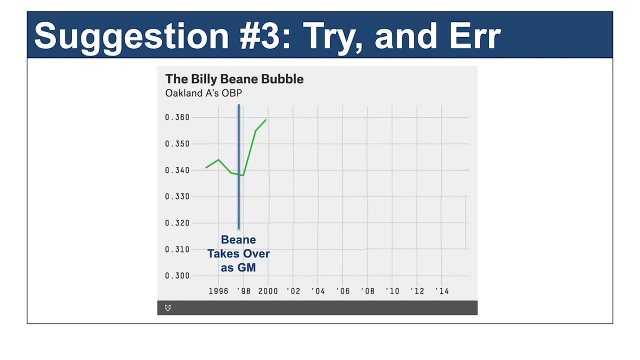 that correlates very well with run scoring. Scoring runs correlates with winning games. Winning games means you win the World Series, although A's never did that, but you get the point right. So this is kind of the story of Moneyball, where Billy Bean takes over the A's. 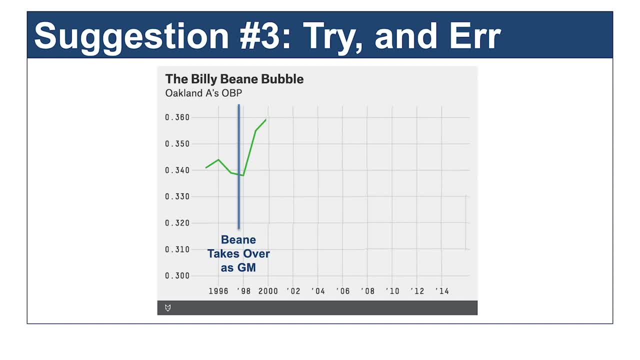 take over and the A's take over. So what you don't hear in Moneyball is the aftermath where, all of a sudden, the A's OBP kind of the year after Moneyball is written begins to plummet down toward revert, toward the mean. So what's happening there? Well, number one, 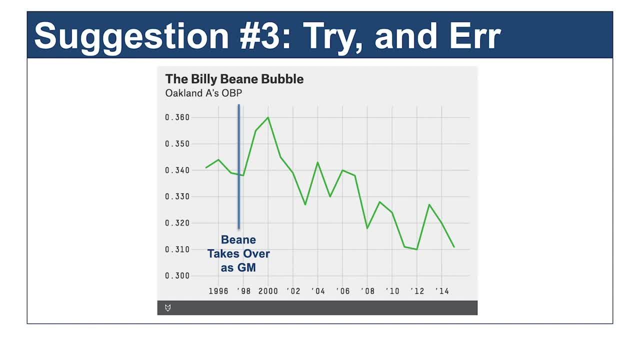 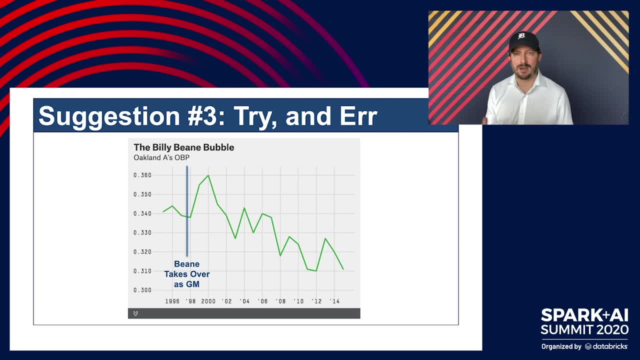 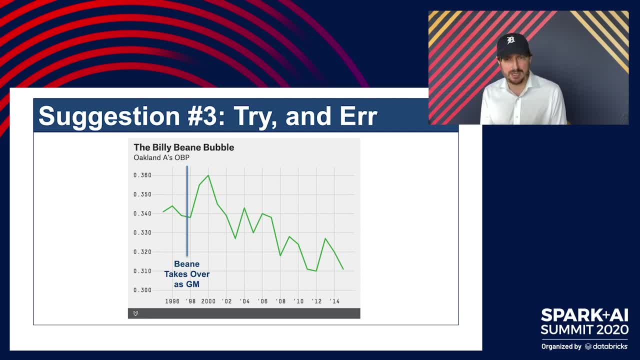 It usually doesn't last for very long. So in the case of the A's, people are like: hey, actually you know what? Billy Bean is right that focusing on OBP is a great way to build up a baseball team. But hey, we're the New York Yankees, the Boston Red Sox. 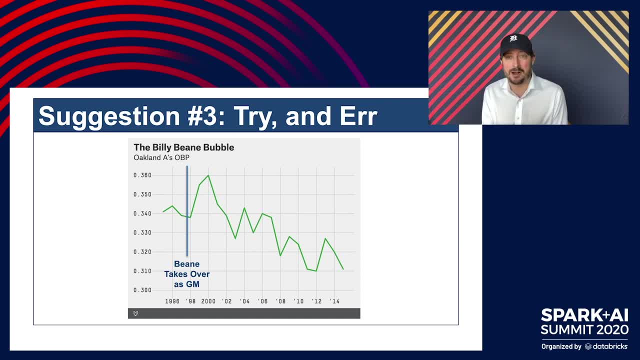 Chicago Cubs- not the Tigers, unfortunately, as much. But we have lots and lots of money and we can copy the A's analytics And therefore we're going to have dominant teams that win 105 games every year, where the A's go back to being a small market team instead. Also realize that. 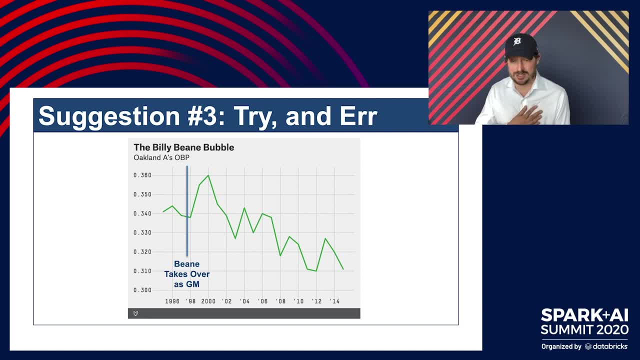 hey look, if you're a pitcher, you don't want to give up walks. It's a valuable intuition as well, And so the market adapts and evolves. You don't always get to be on that early part where the learning and the growth is very steep. With that said, there is a lot to be said for improving. 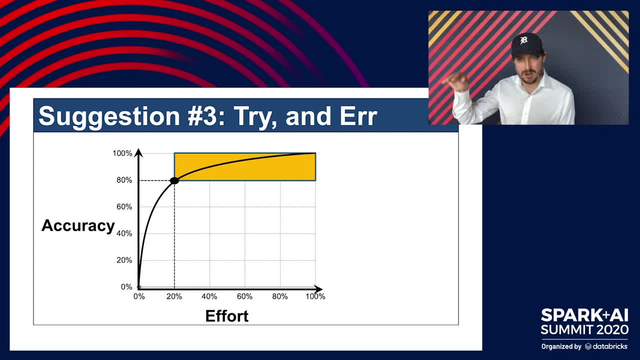 incrementally along the margin and making marginal gains 1% of the time, or 0.1% of the time Every year, when we build our election model, what I've been working on for the past few weeks. we could have just taken our 2016 model off the shelf and applied it. We're actually very 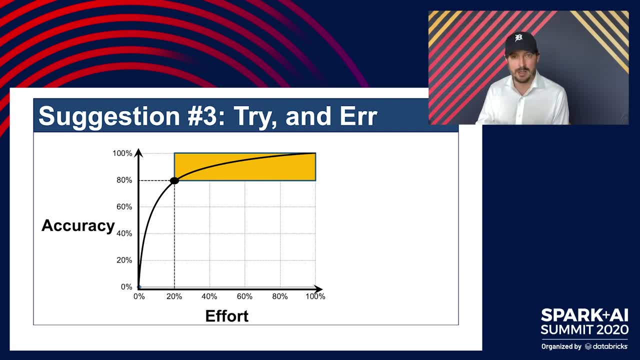 proud of that model. I think it did a good job to give Trump a better chance than the convention of Winston or the other forecasted. But still, I like to rebuild my models every time. we do them because you're learning a little bit at a time And I believe that, hey look, we are getting the 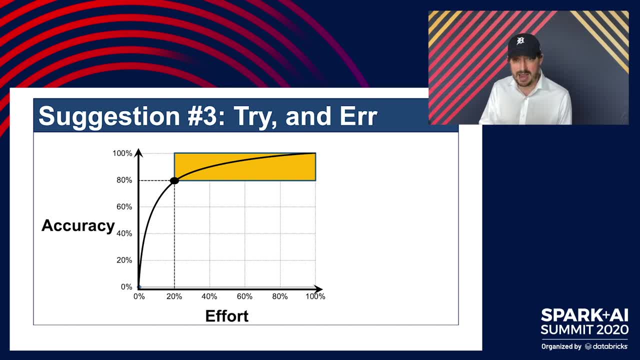 big stuff. right, we think, but making a little improvement about how you analyze different types of polls. What happens when you have polls that seem to contradict one another? How do you measure the economy during a time of coronavirus? All those marginal improvements are often where in a competitive environment. you're going to be able to do a lot of things. You're going to be able to do a lot of things. You're going to be able to do a lot of things. You're going to be able to. 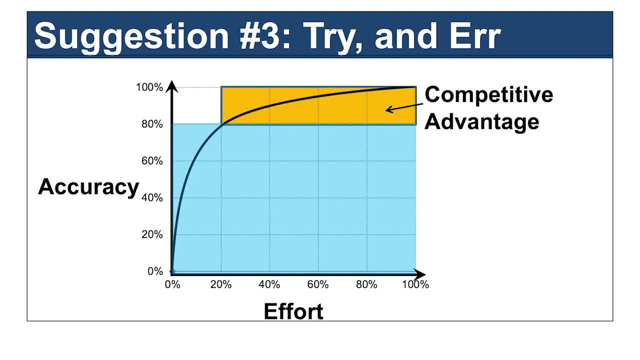 in a competitive environment that you really differentiate yourself from. Again, it's great when you're an early adapter. you have an idea that no one else has really been able to apply at scale. Unfortunately, it might only happen a couple of times in your career or your company's. 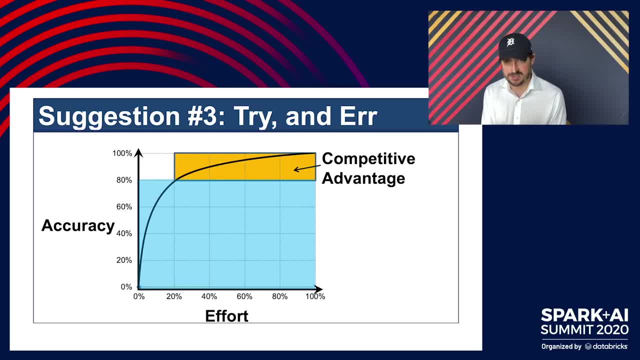 lifespan. You instead have to make continuous improvement around the margin. So again, I'm saying that making small, marginal, incremental improvements is often the name of the game, and these are things that you should be mindful of. One thing about Bayes' theorem, by the way, is that there's never actually an endpoint in Bayes'. 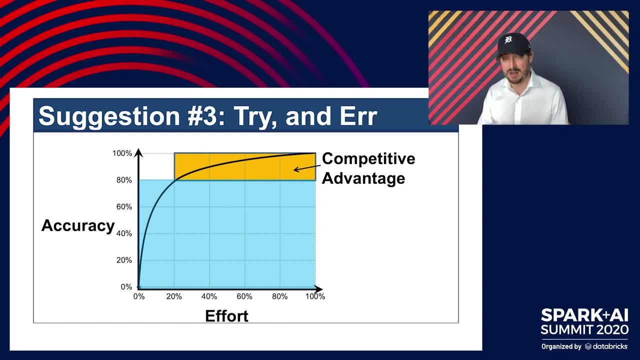 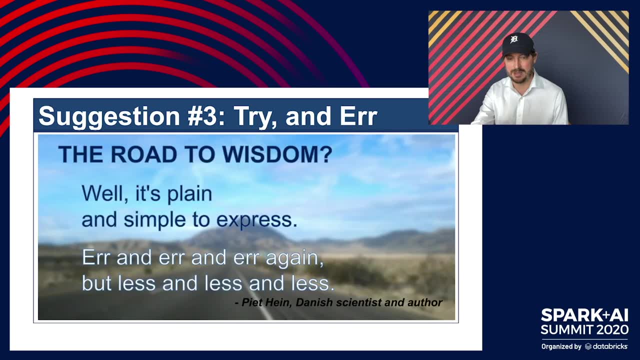 theorem. You start out with a belief, you collect evidence, you refine and revise that belief and you get a little bit better over time, And it's a process of continued improvement. So I'll kind of sum up with this poem. I guess it is from Piet Hein, who is a Danish scientist and